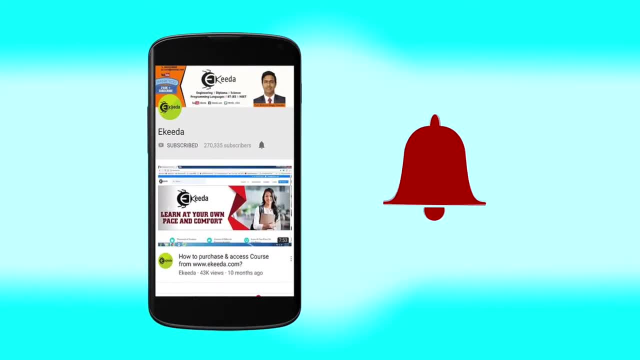 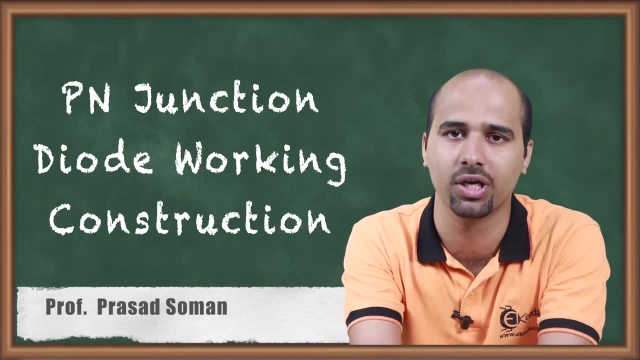 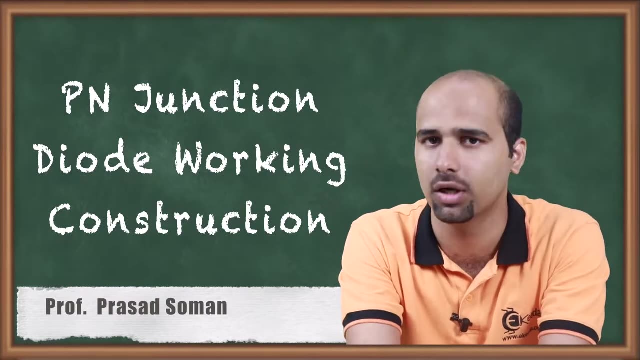 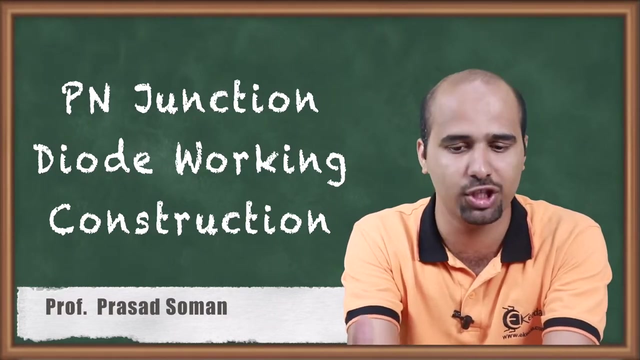 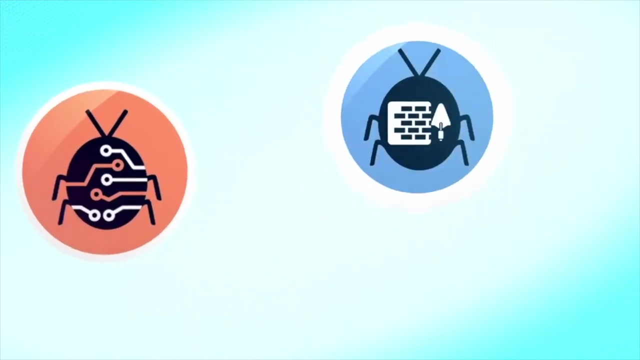 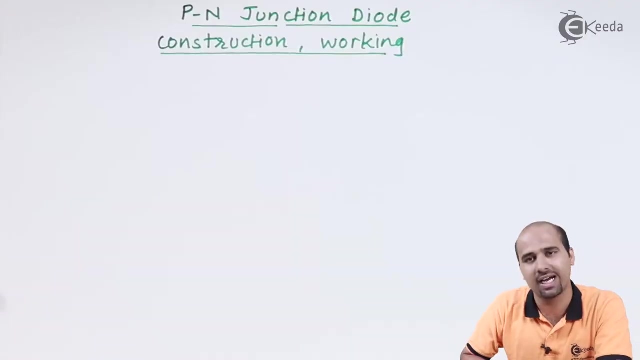 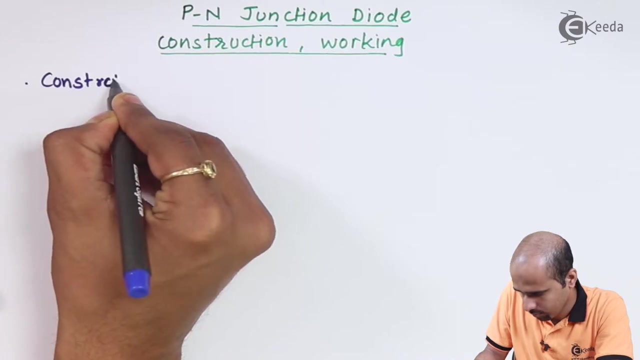 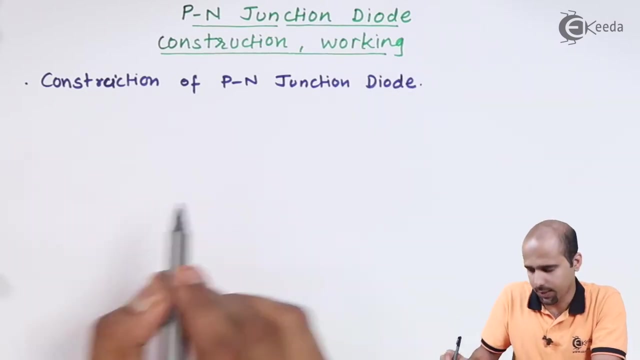 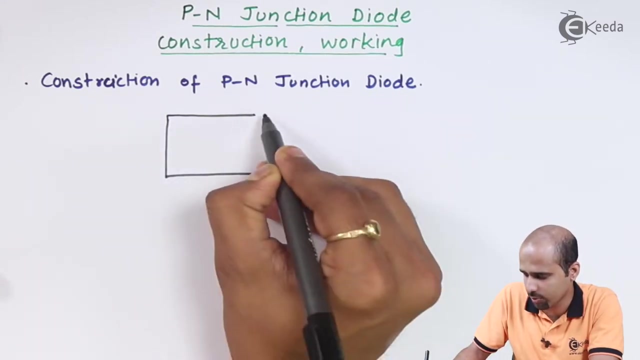 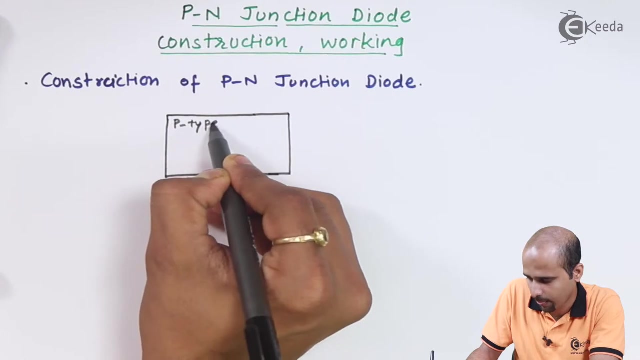 Click the bell icon to get latest videos from eKIDA. So let us start with the construction of p-n junction diode. first See in the last video lecture. I have taken one simple rectangular box. I have named this as p-type of semiconductor, isn't it? 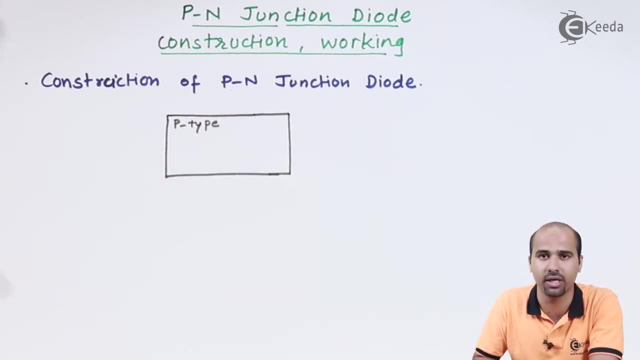 In this p-type of semiconductor. I know that in the p-type of semiconductor all the majority charge carriers are nothing but the holes. So the charge carriers are nothing but the holes. So the charge carriers which are responsible for the conduction process are nothing but. 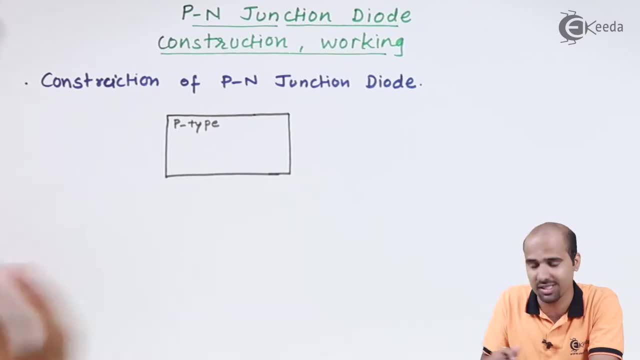 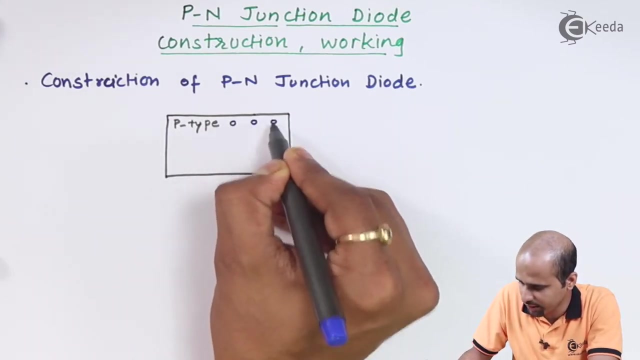 the holes. But don't think in that way. even though this is p-type semiconductor, I will not be having any electron as a carrier. No, I will be having few minority charge carriers as well. So we will be having few minority charge carrier as well as, majorly, I will be having majority. 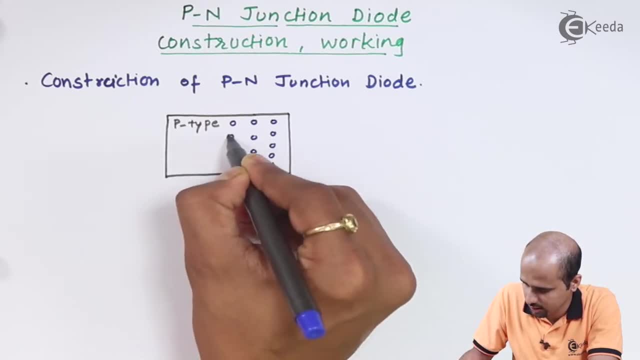 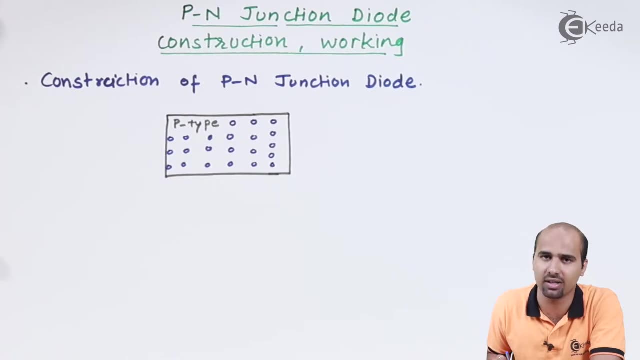 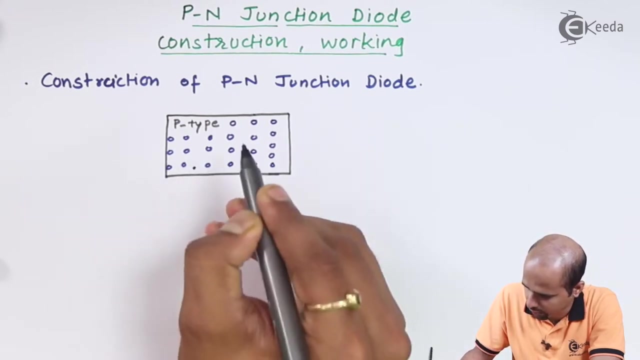 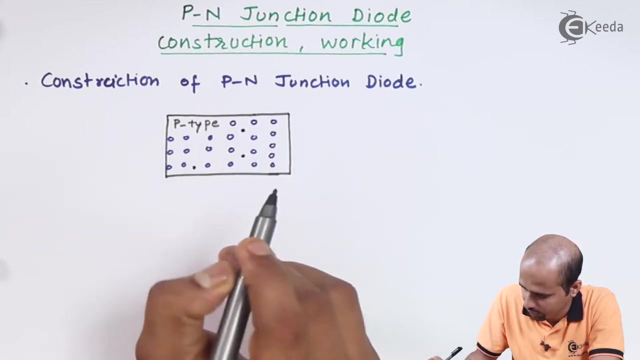 charge carrier as whole. So this is p-type. All these rounds are nothing but the positively charged carriers. that are nothing but holes. I will mark these points. Black points are nothing but few black points. I have mentioned only three amongst all these around 20-25 holes. 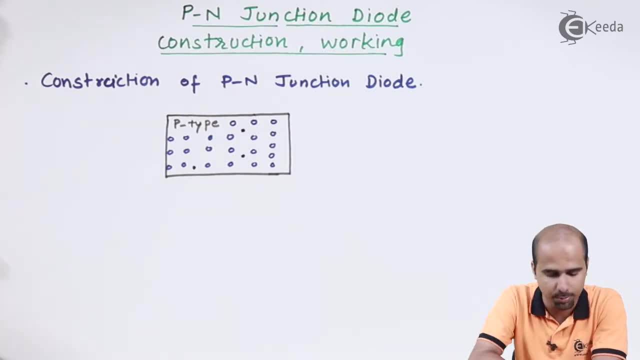 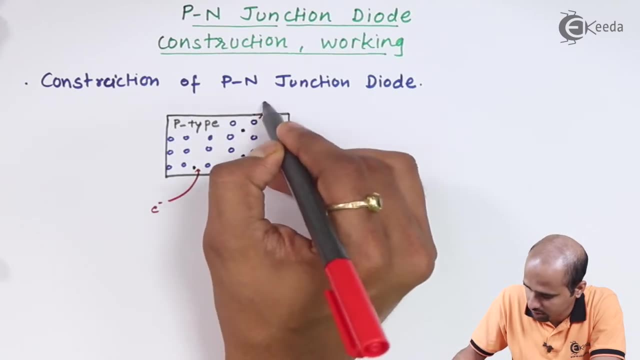 So these three points are nothing but electrons, called as a minority charge carriers. So we will say we will do for that. This is nothing but the electron. So we will do them nothing but the electrons. and these are nothing but the holes. So same story, we will repeat. 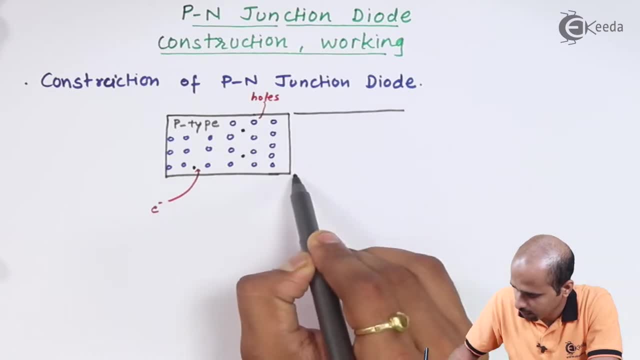 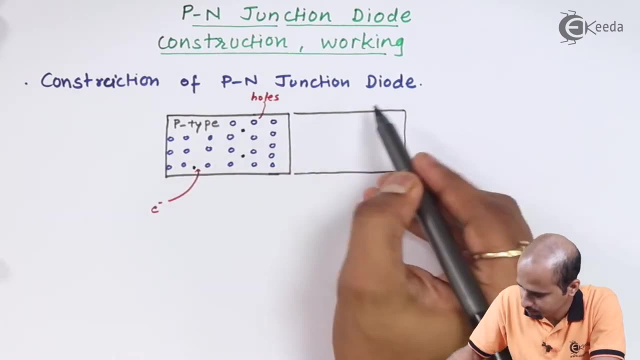 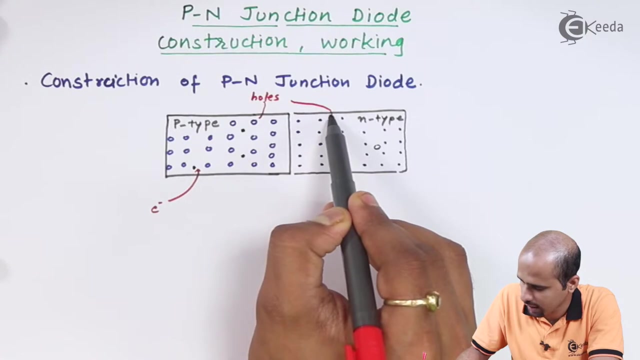 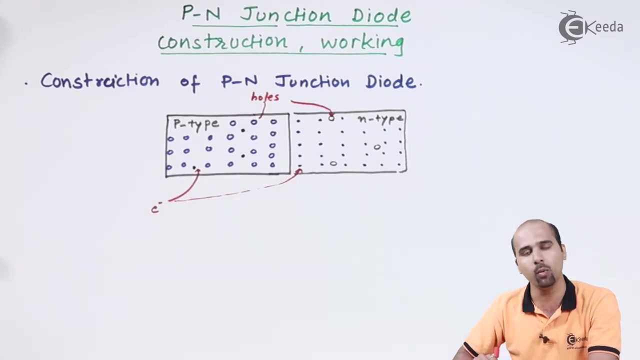 for n type of semiconductor. For n type of semiconductor, the story is exactly opposite. So here we will be having holes as minority charge carriers and electrons as majority charge carriers. Now, what will happen if I combine them? This p type is having holes. These 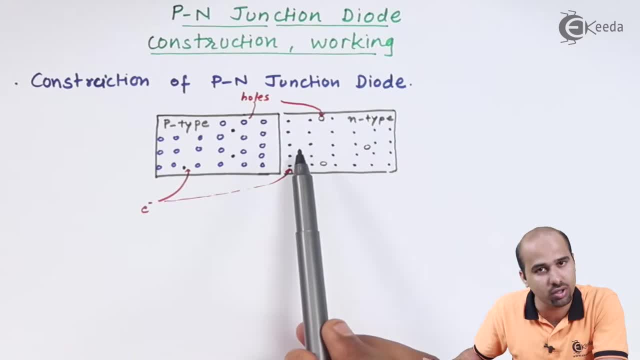 are positively charged carriers. This n type is having electrons. These are negatively charged carriers. As far as Coulomb's law of electrostatics, we all know that positive and negative may pyaar hota hai. So what will happen? This negatively charged electrons will jump towards the positively charged holes and 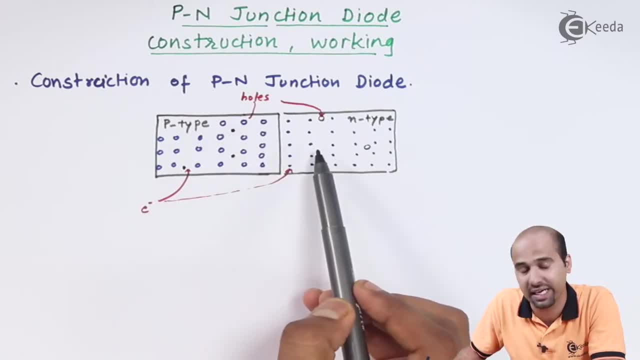 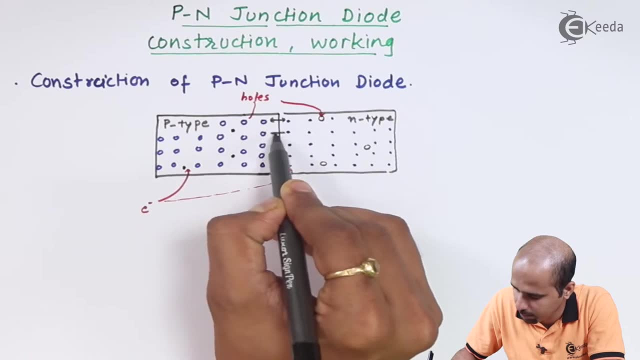 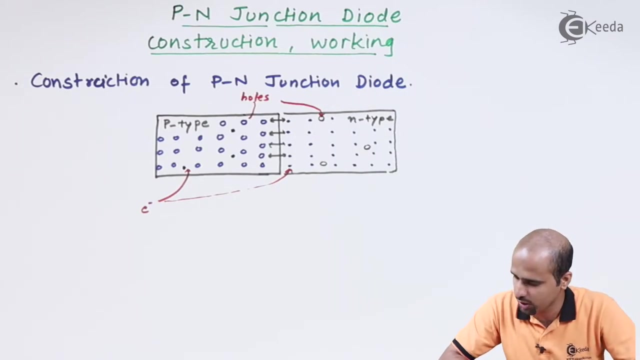 positively charged holes will jump towards the negatively charged electrons. So what will happen? These electrons and holes will get recombined. And what will happen after recombination, When electrons will move from n type to p type substrate? then what will happen Here? 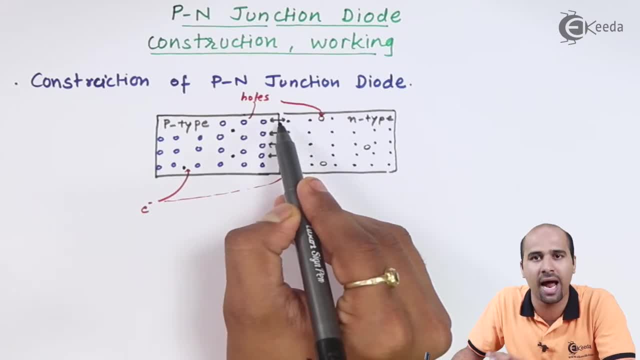 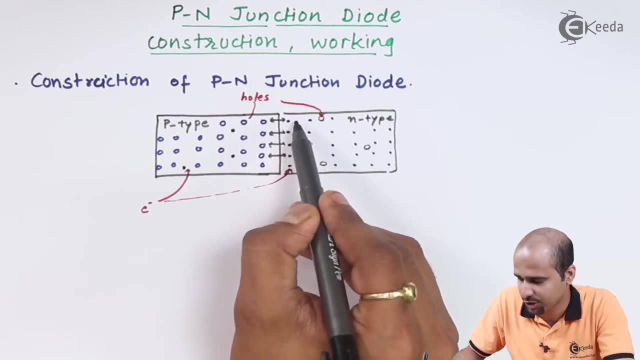 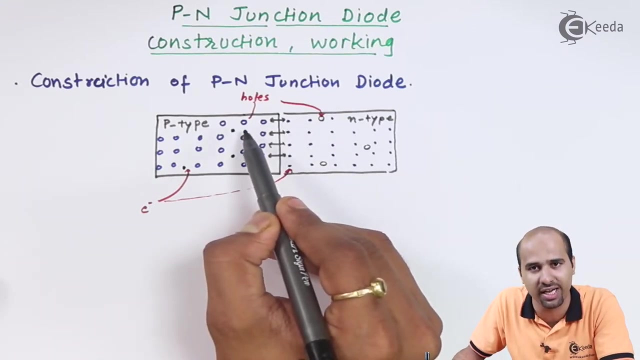 I will be getting one ion. Atom is converted into ion. This is because one electron is left from that atom and due to that I will be having one positively charged ion, because ek electron chhod ke chala gaya, so dominance is in the form of positively charged. So 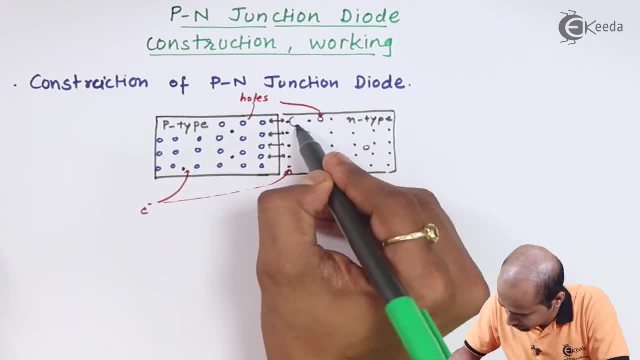 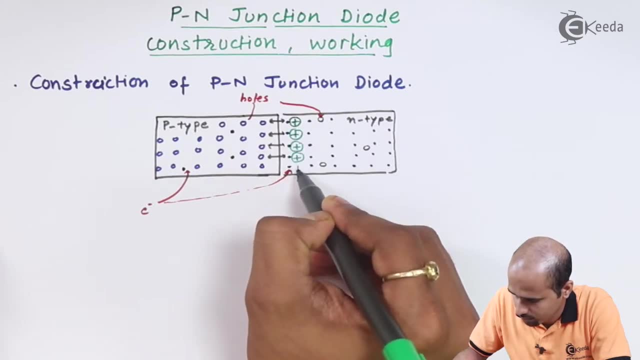 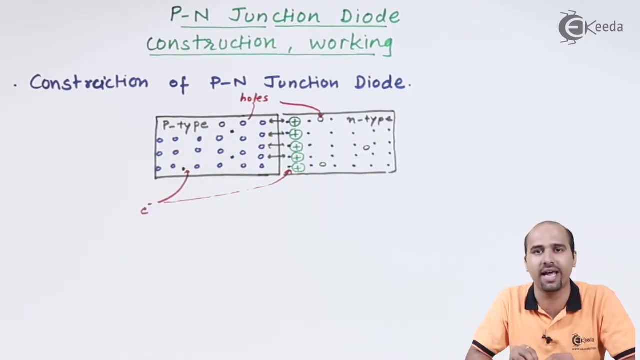 what will get? We will be getting one extra positively charged ion 5.. This is the point. Similarly, if this hole is having one extra electron added into that particular atom, Atom gets converted into ion, But in this particular process, one extra negatively charged. 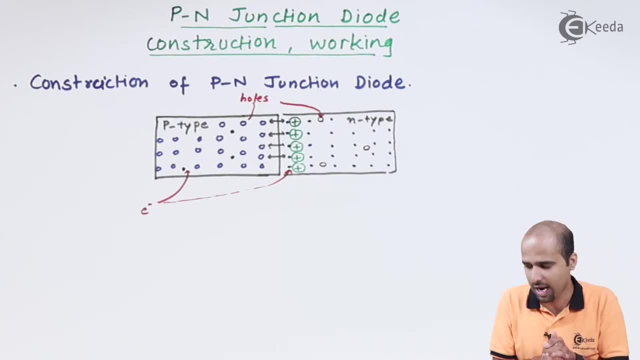 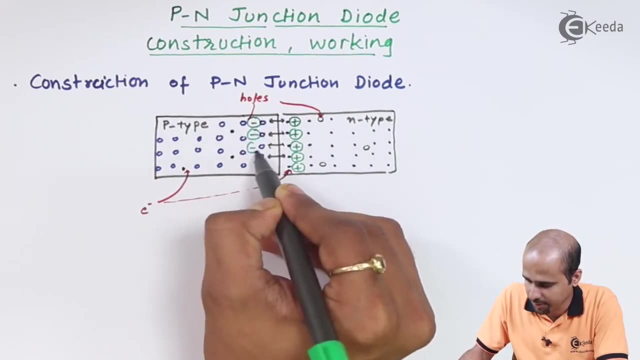 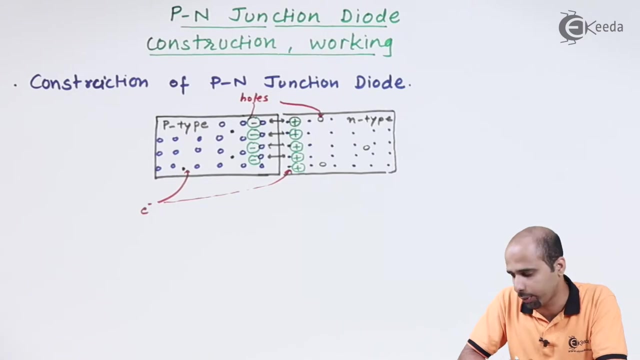 carrier is acquired in that particular Atom. SO THIS ATOM is of the form of negatively charged ion, FUTURE CARRIER. So atom gets converted into ion. that is nothing but the negatively charged ion. Now, after that, what will happen? these all electrons are also there. all the electrons will try to jump towards. 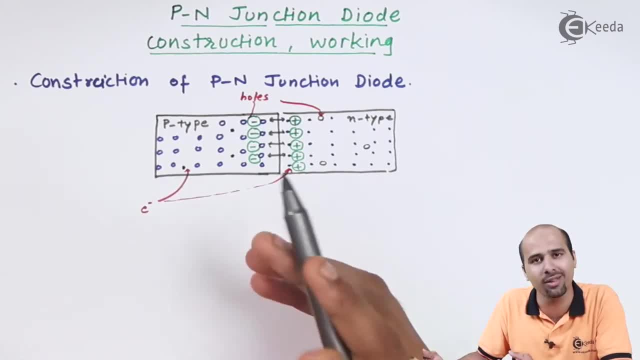 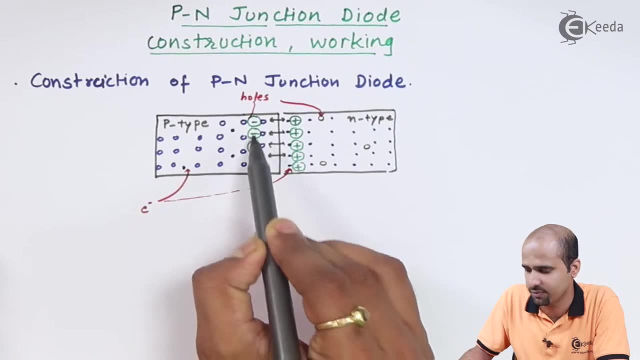 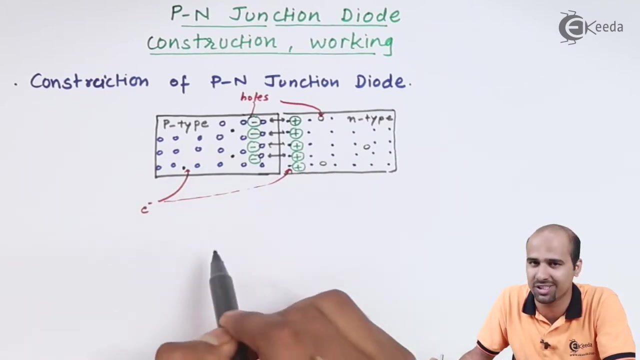 the p-type semiconductor, but all the electrons are not allowed to move towards the p-type semiconductor. this is because these are ions which are negatively charged carriers and, again, according to Coulomb's law of electrostatics, negative. negative may dushmani hoti hai positive. 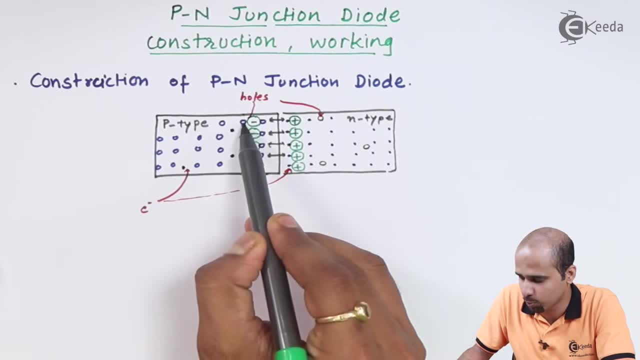 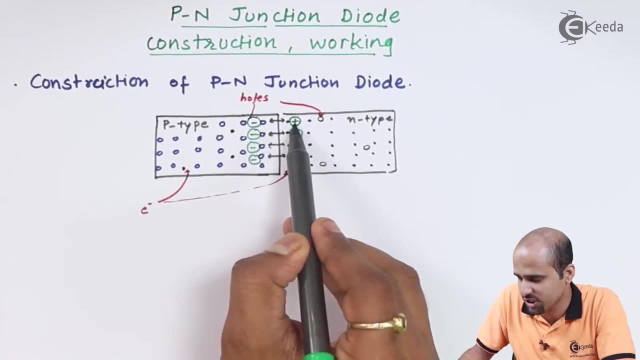 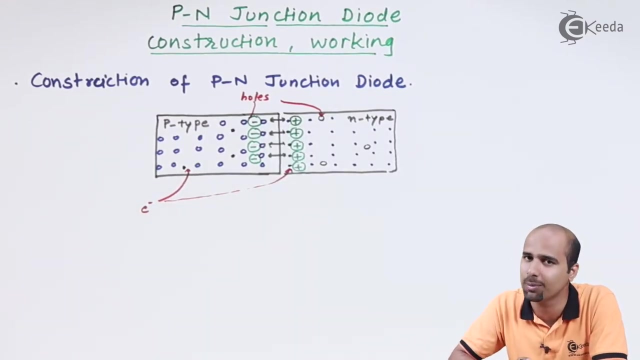 positive may dushmani hoti hai. even if I try to move this holes, even these holes try to move there themselves towards the n-type. these positively charged ions will resist themselves. so what will happen? electrons which are having sufficient amount of energy to move to cross the 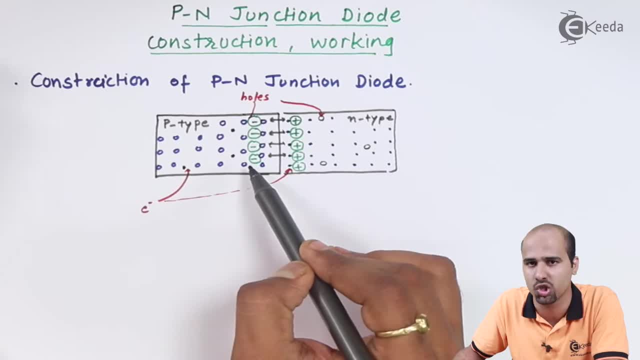 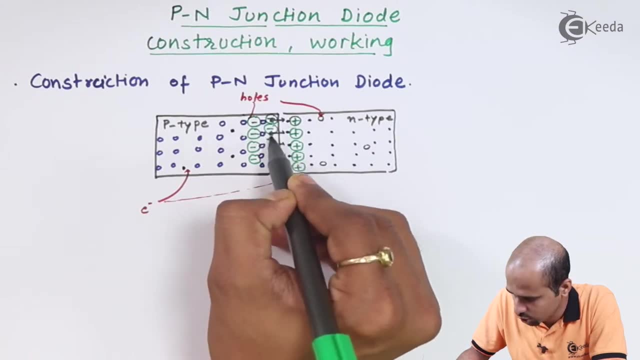 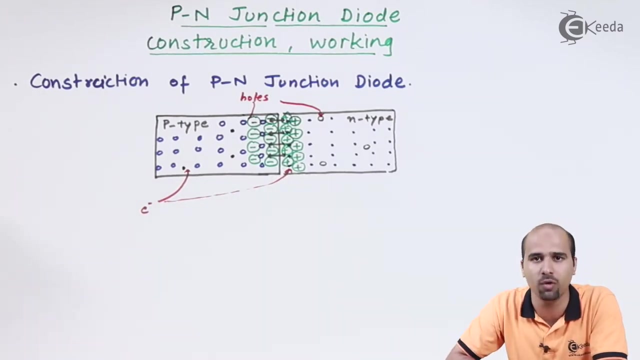 barrier of these ions. only those electrons will recombine with the holes right. so I will say that all the electrons are recombined so that I will get the positively charged ions. so as many number of positively charged ions I will be getting and negatively charged ions I will be getting depends on the number of recombinations. 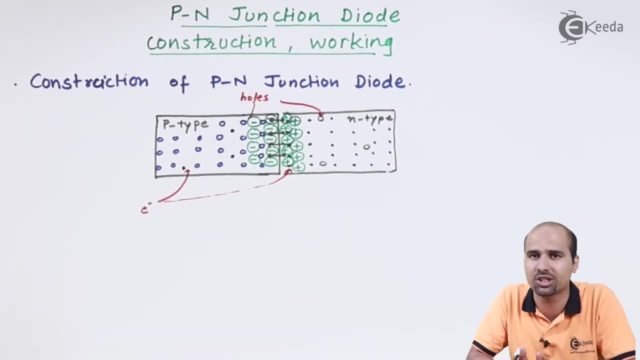 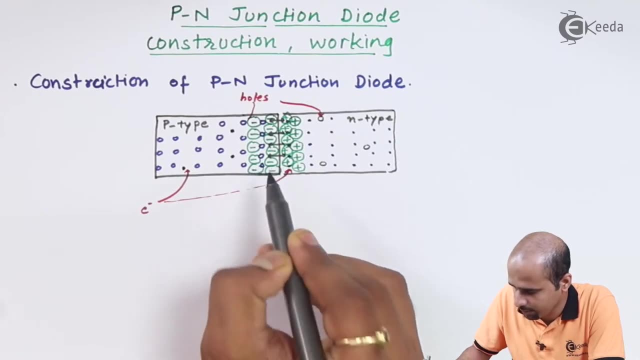 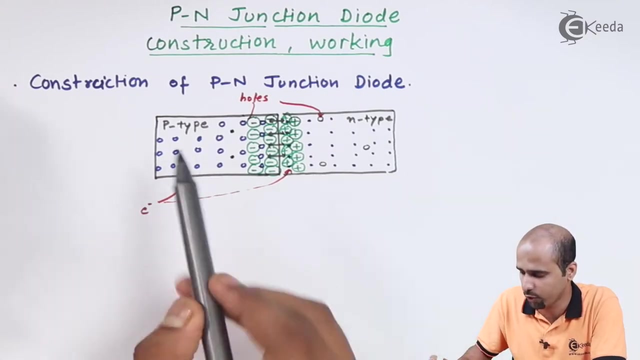 jitna, recombination, badega utna hi junction me resistance, badega right. so at one particular level, what we can do is we can say that here i will be having complete wall which is improving, increasing resistance to move from p-type to n-type for holes and n-type to p-type for electrons. now 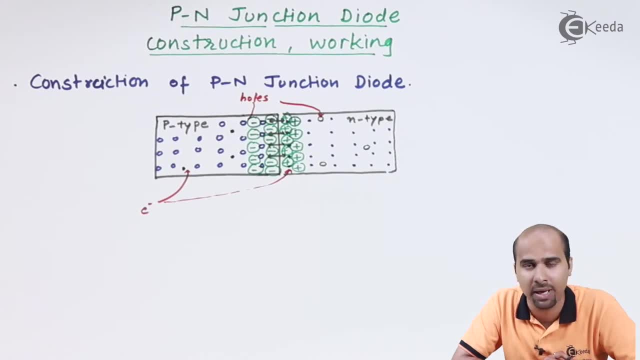 here after it is not possible for electrons to move towards speed type and holes to move towards the n-type. this complete process is called as diffusion. the movement of electron from n-type to p-type and holes from p type to n type, which forms the barrier, is called as diffusion. so the process 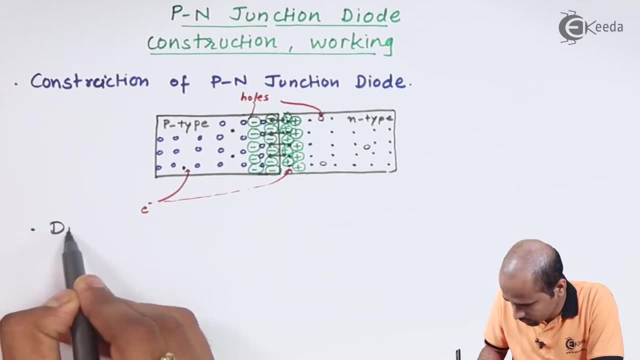 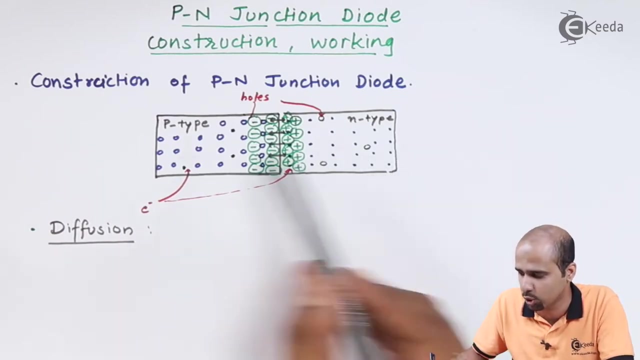 is nothing but diffusion, mind well, the beauty of that diffusion is i just recombine the holes and electron without applying any external potential. i haven't applied any external wiring circuit over there to push themselves into one for one region to another region. no, it is not necessary, right. 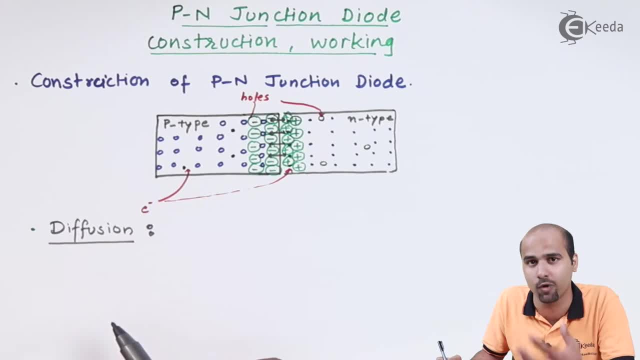 so that's why it is called as diffusion. they themselves form the movement from n type to p tap and p type to n type, so this is called as diffusion. now another process that is called as drift. people many times get confused between these two concepts. mind well, diffusion is the process in 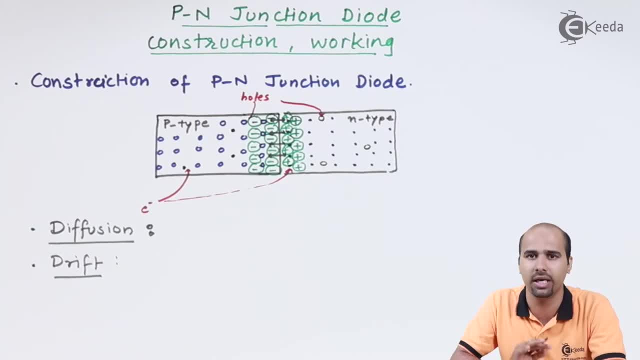 which, without any external potential, electrons move from n type to p type and holes move from p type to n type to form a barrier that is called as diffusion. when i'm going for drift, drift is nothing but the process in which the, the, the, the, the electron moves from n type to p type and holes moves from p type to n type. after applying 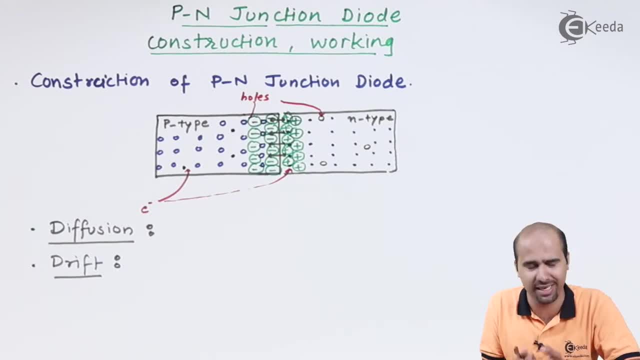 external potential or external energy. that energy may be in the form of electrostatic energy, may be in the form of magnetic energy, may be in the form of thermal energy or any kind of energy. generally in our syllabus, generally in our circuits, we use one particular extra potential supply so that with 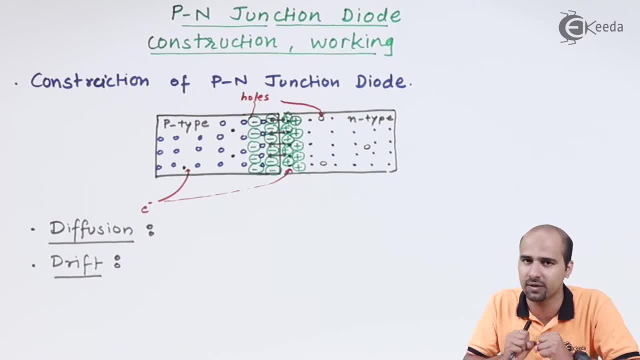 that positive and negative energy supply we can get a positive energy supply so that with that positive and negative potential we will be getting the force to move electrons towards the p type and holes towards the n type. that process is called as diffusion. let us come to the point that is working. 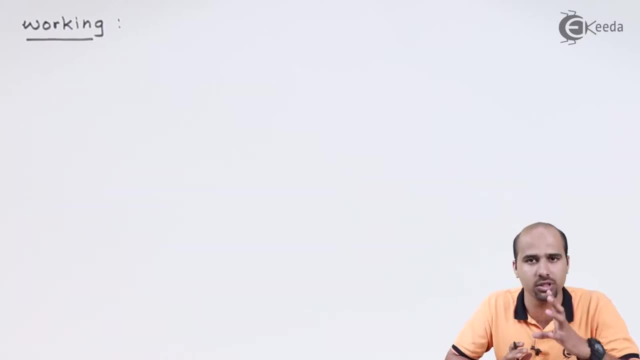 of this particular diode. first point: may we have discussed that how the electrons moves from one region to another region to form the diode. now i have formed the diode before going towards the working diode, before going towards the working diode, before going towards the working diode. 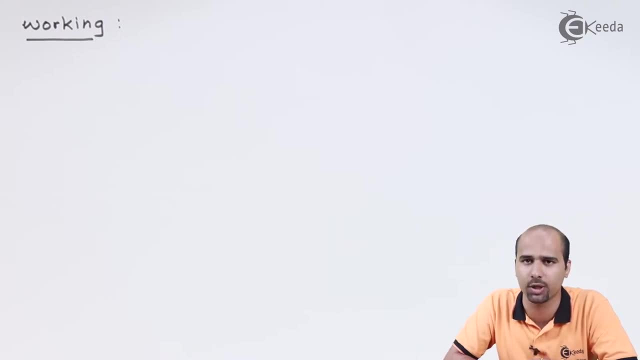 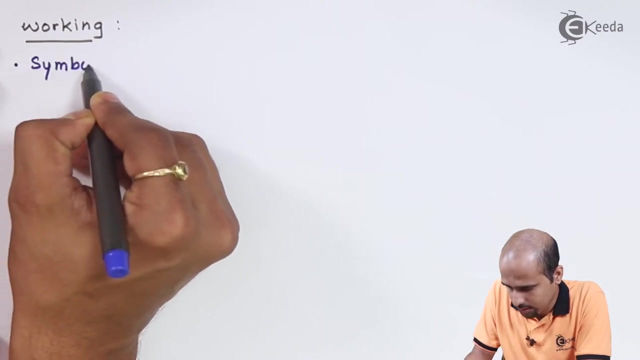 we have to know that how we will represent the diode. is it possible to represent the diode with two boxes of n type and p type every time? no, it is not necessary. it is not possible as well. so what we will do, we will first go for the symbol. symbol of diode is nothing but. 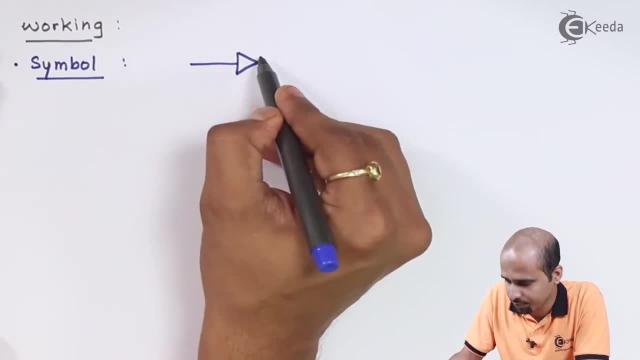 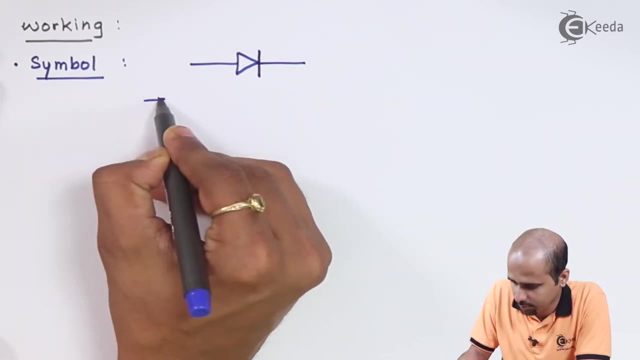 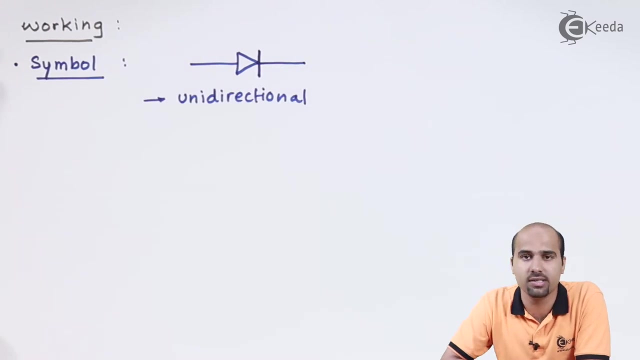 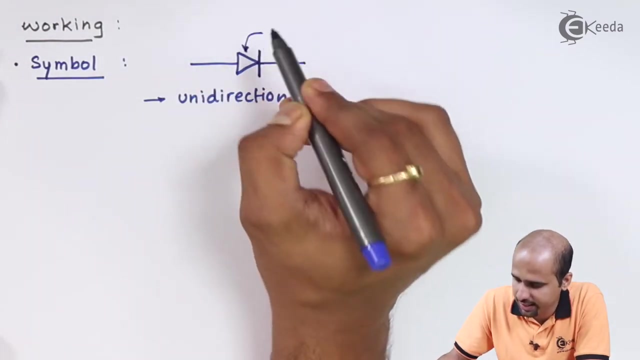 one arrow, that is triangle, and one line, which shows that this diode is nothing but unidirectional. what do you mean by unidirectional? there is the flow of current which is possible in only one direction, and this direction is decided by this arrow. arrow represents direction. 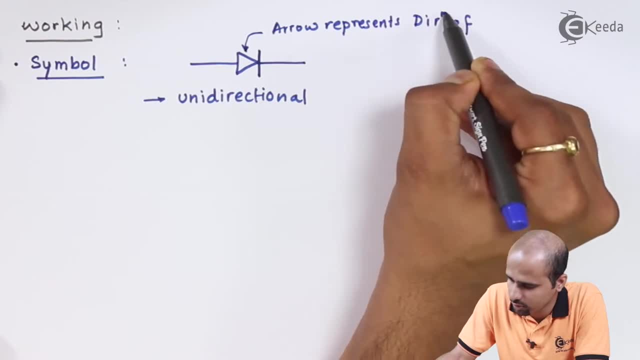 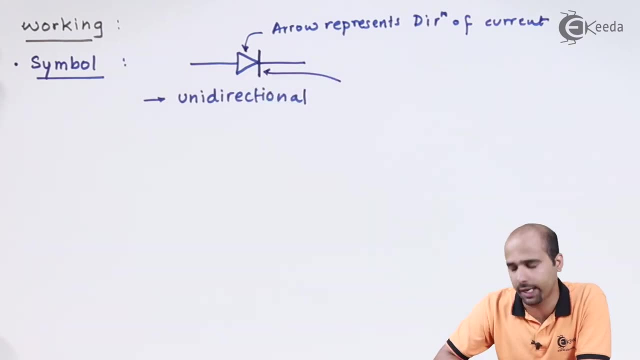 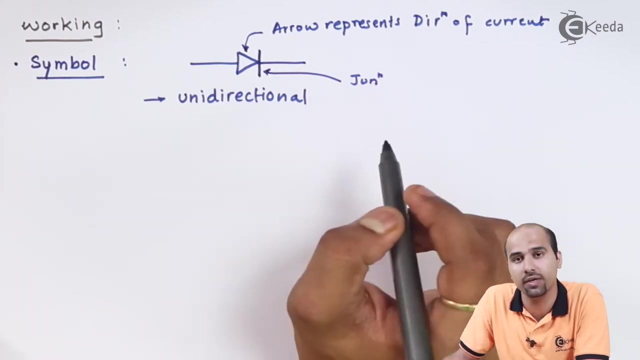 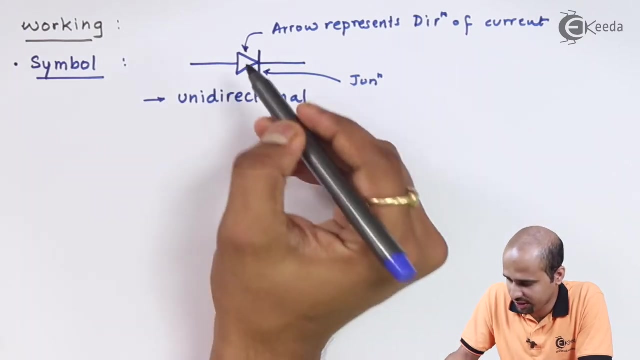 direction of current, and this vertical line represents the junction or barrier which is getting formed with the diffusion process. so, whatever formation of this device is called as pn junction diode. so let us move towards the process of working. so let us move towards the process of working. 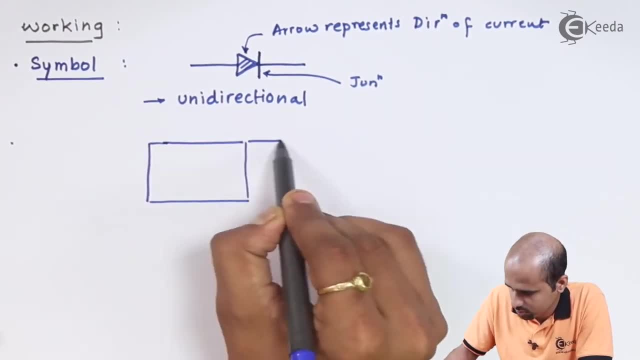 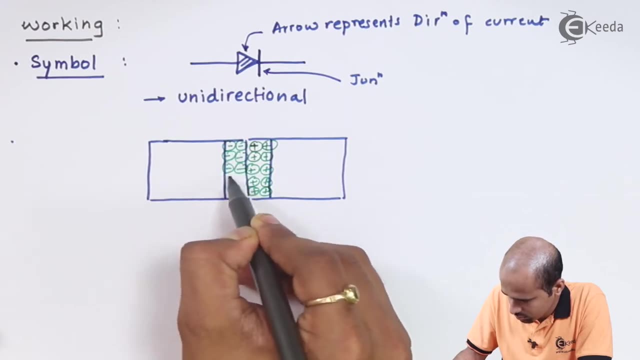 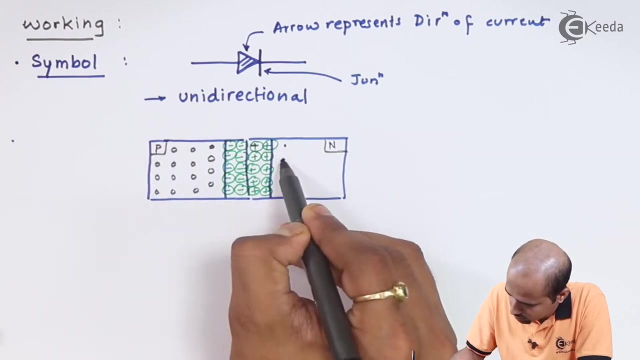 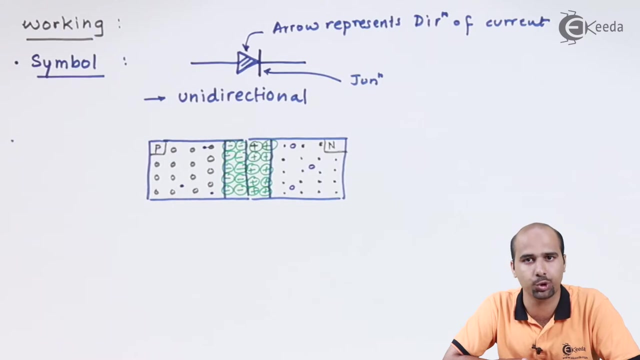 so this is how the diode is getting formed after the diode is getting formed after the diode is getting formed after the process of diffusion. so what will happen with the internal potential with this particular junction of the diode? this junction is having one potential difference. this is because 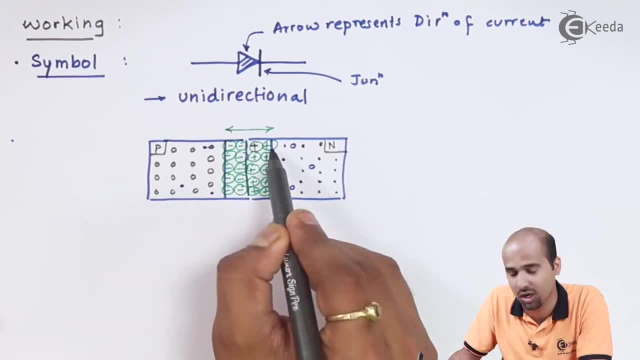 this is of negatively charged potent ions. this is of positively charged ions. so there will be a fixed potential difference between the junction in between, the junction from n type to p type. so there will be a fixed potential difference between the junction in between the junction from n type to p type. 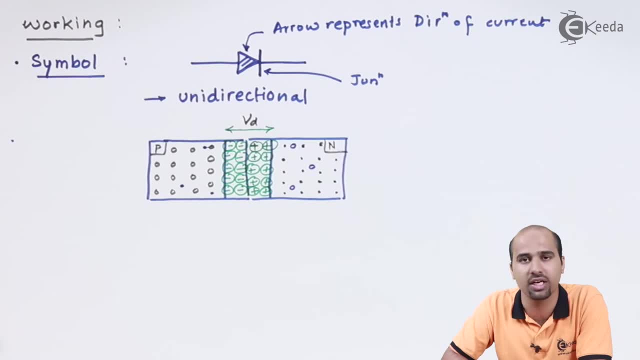 so whatever potential i will be getting, that is called as junction potential. so this is denoted by vd. so whatever potential i will be getting, that is called as junction potential. so this is denoted by vd. so whatever potential i will be getting, that is called as junction potential. so this is denoted by vd. vd is called as: 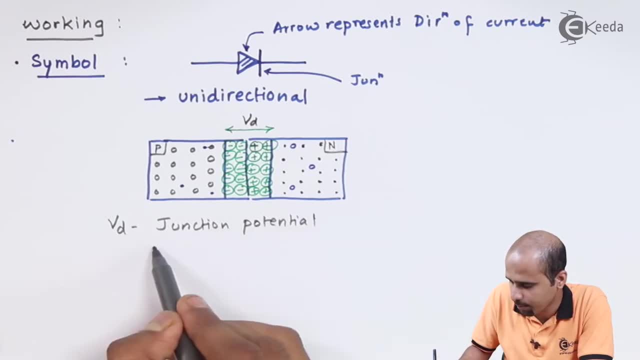 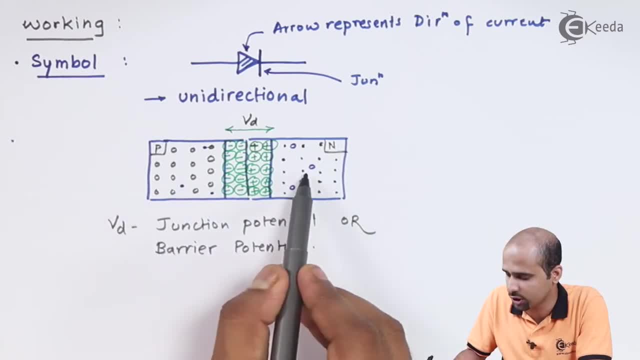 difference. then and only then it is possible to difference. then and only then it is possible to form a barrier between the electrons in the form, a barrier between the electrons in the form, a barrier between the electrons in the n type and holes in the p type. n type and holes in the p type. 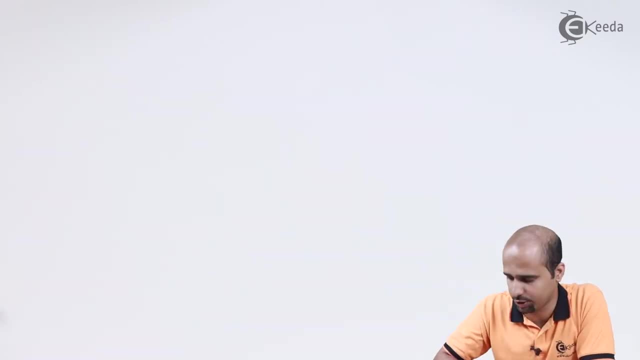 n type and holes in the p type. now we will form the working in the form. now we will form the working in the form. now we will form the working in the form of drift operation, in the drift operation of drift operation, in the drift operation of drift operation in the drift operation. we will be having two. 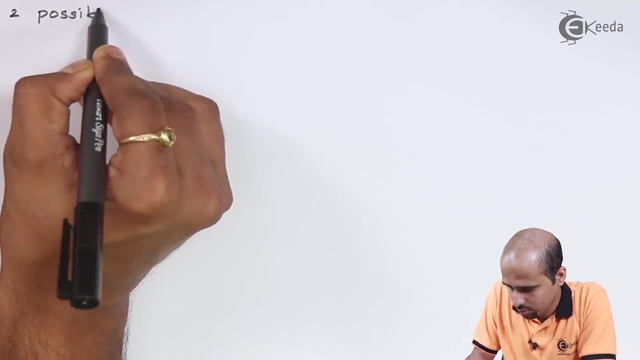 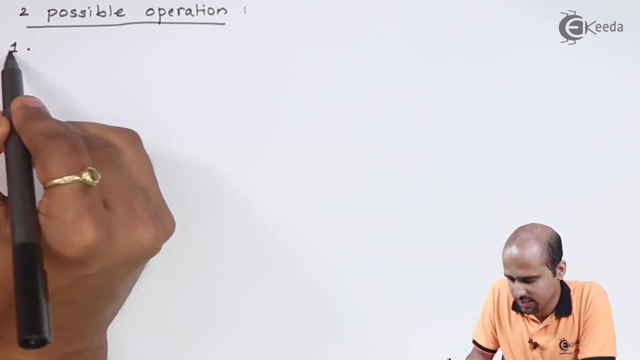 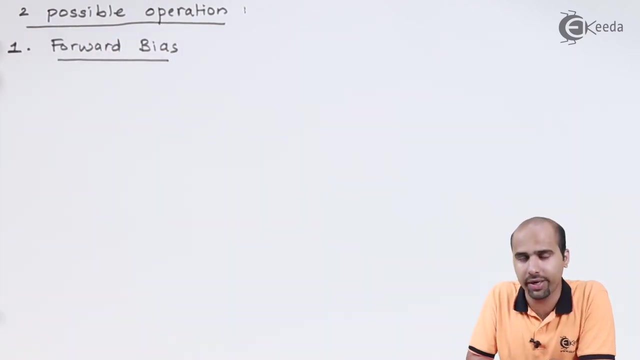 we will be having two. we will be having two possible operation, operation operation. one is called as forward bias and another is one is called as forward bias and another is one is called as forward bias and another is called as reverse bias. called as reverse bias, called as reverse bias. again, we will repeat this particular circuit. 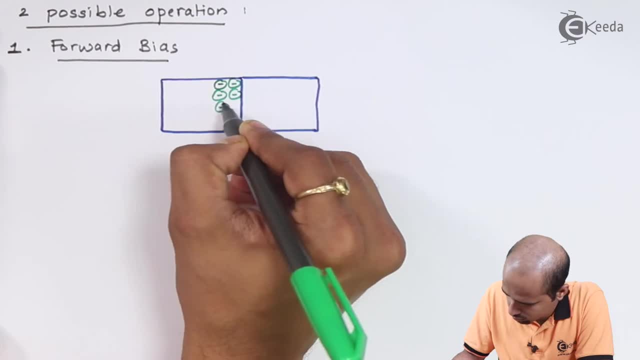 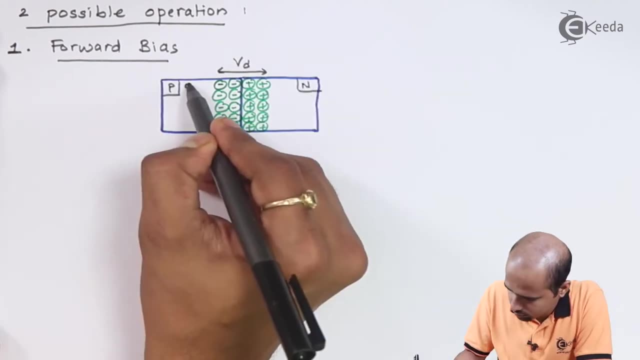 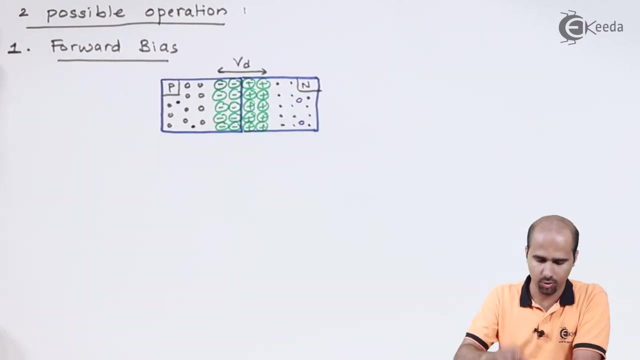 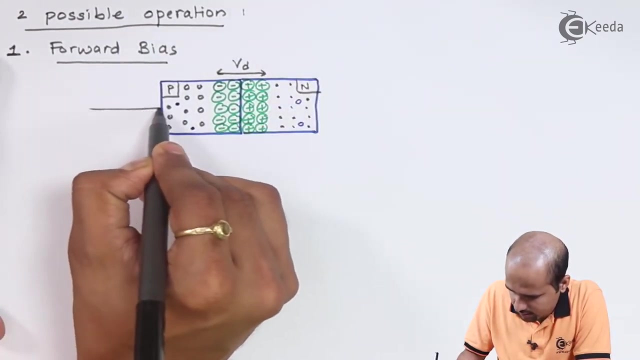 again, we will repeat this particular circuit. again, we will repeat this particular circuit. okay, this is a simple diode, okay. okay, this is a simple diode, okay. okay, this is a simple diode, okay, now, now, now, with this we will form, with this we will form. 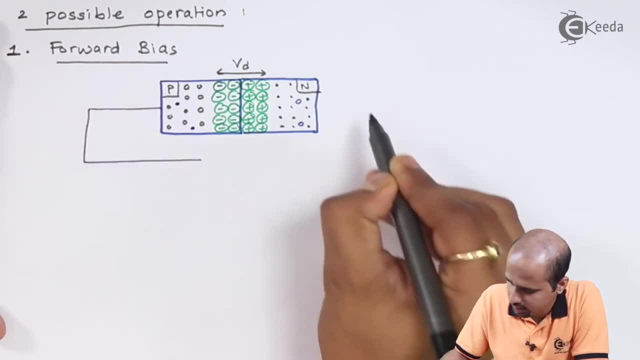 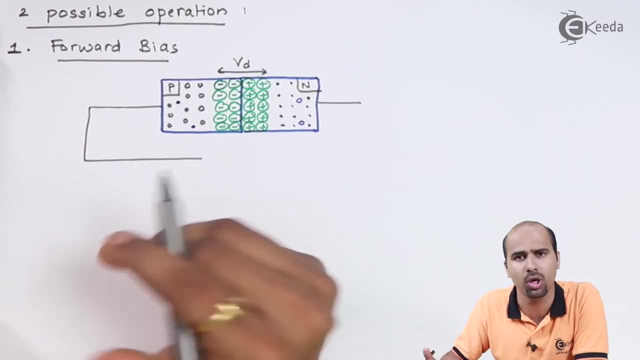 with this, we will form the external circuit, the external circuit, the external circuit, such that, such that, such that i will get the external force for the, i will get the external force for the, i will get the external force for the electrons to move towards the p type or 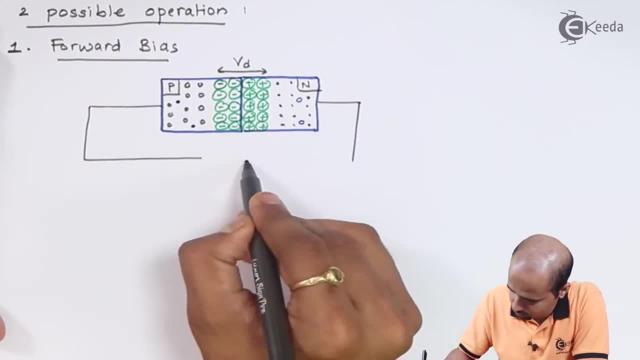 electrons to move towards the p type, or electrons to move towards the p type, or holes to move towards n type holes to move towards n type holes, to move towards n type, as we have learned in pre-requisite, as we have learned in pre-requisite, as we have learned in pre-requisite session. 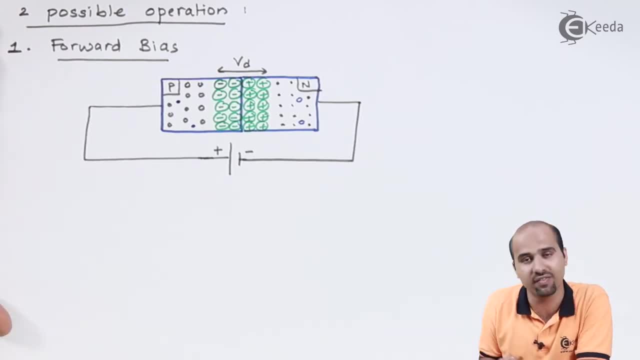 session session. what are the dc and ac sources here we? what are the dc and ac sources here we. what are the dc and ac sources here we have applied, have applied, have applied dc source. so this dc source represents dc source. so this dc source represents dc source. so this dc source represents that. this is my negative potential and 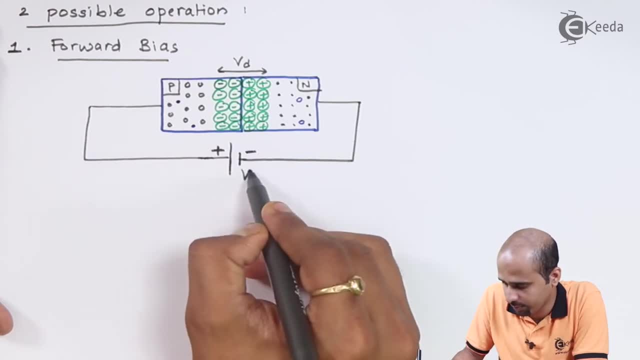 that this is my negative potential and that this is my negative potential and this is my, this is my, this is my positive potential of battery v. positive potential of battery v. positive potential of battery v. so so so, let us start with the operation if i am. let us start with the operation if i am. 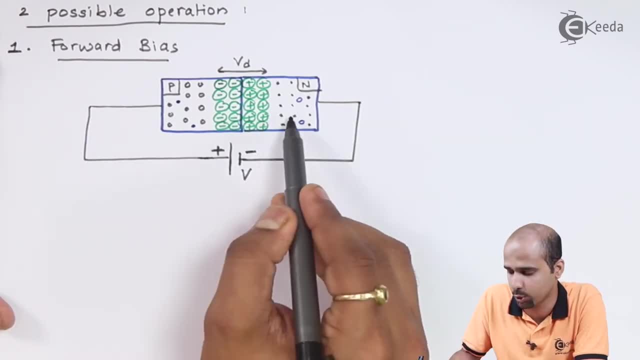 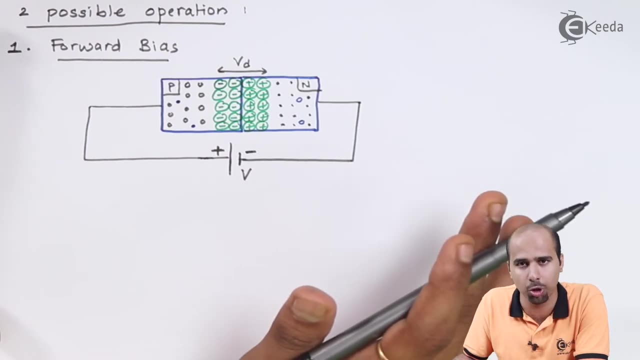 let us start with the operation. if i am talking about this negative terminal, of talking about this negative terminal, of talking about this negative terminal, of what will happen. what will happen, what will happen according to electrostatics law coulomb's. according to electrostatics law coulomb's. 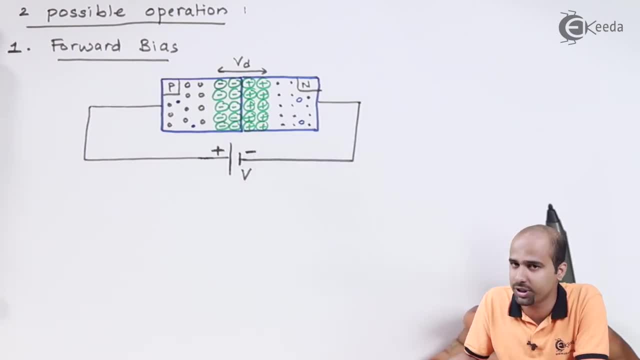 according to electrostatics law, coulomb's law of electrostatics, law of electrostatics, law of electrostatics, the negative, negative, so we can say that the electrons, so we can say that the electrons, so we can say that the electrons will not enter into the negative part. 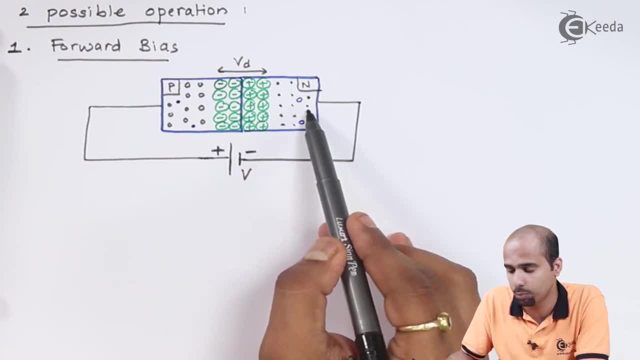 will not enter into the negative part, will not enter into the negative part of the battery, rather than that these of the battery, rather than that these of the battery, rather than that these electrons, electrons, electrons will move away from that negative, will move away from that negative, will move away from that negative potential. that means 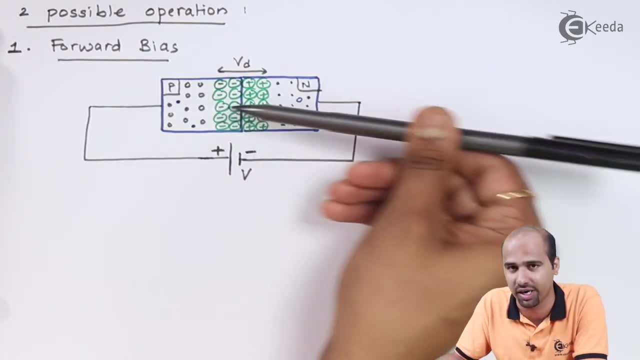 potential. that means potential. that means these electrons will try to move towards these electrons will try to move towards these electrons will try to move towards the junction right. so electrons will get the junction right. so electrons will get the junction right. so electrons will get force to move towards the junction. the 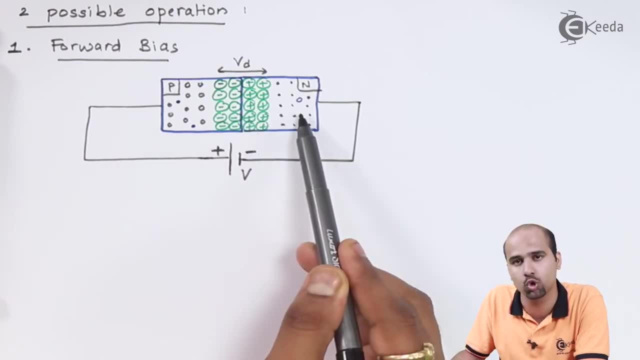 force to move towards the junction, the force to move towards the junction, the amount of energy the electrons will get. amount of energy the electrons will get. amount of energy the electrons will get to cross that particular barrier and to cross that particular barrier and to cross that particular barrier, and again it will form, it will recombine. 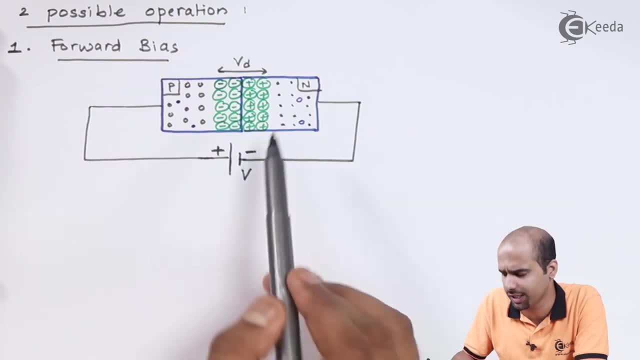 again. it will form. it will recombine again. it will form. it will recombine with the holes. but what will happen if i with the holes? but what will happen if i with the holes? but what will happen if i say that these electrons will recombine, say that these electrons will recombine? 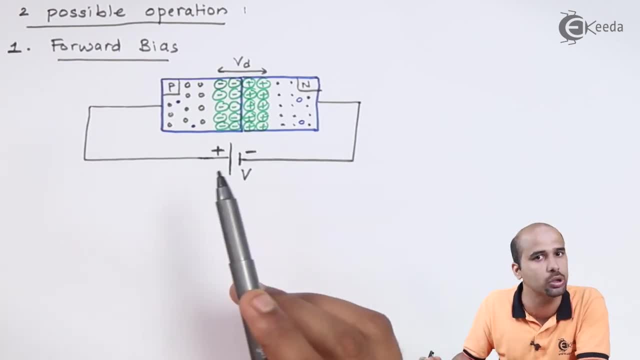 say that these electrons will recombine with the holes, with the holes, with the holes. again, another ion will get formed. this is again, another ion will get formed. this is again, another ion will get formed. this is not so, not so, not so. this is because this positively charged 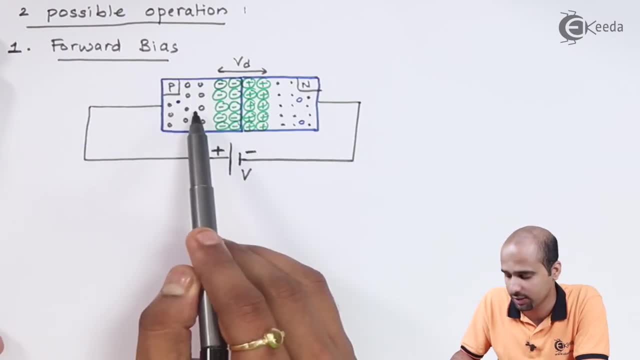 this is because this positively charged. this is because this positively charged carrier, this positively charged carrier carrier, this positively charged carrier carrier, this positively charged carrier, that is whole. that is whole. that is whole. are moving towards the n-type as well. are moving towards the n-type as well. 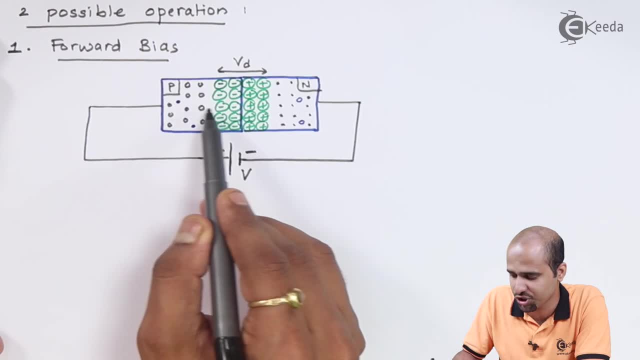 are moving towards the n-type as well, so that's why i am saying that. if so, that's why i am saying that. if so, that's why i am saying that. if electrons are moving here, electrons are moving here. electrons are moving here, getting attracted towards this positive 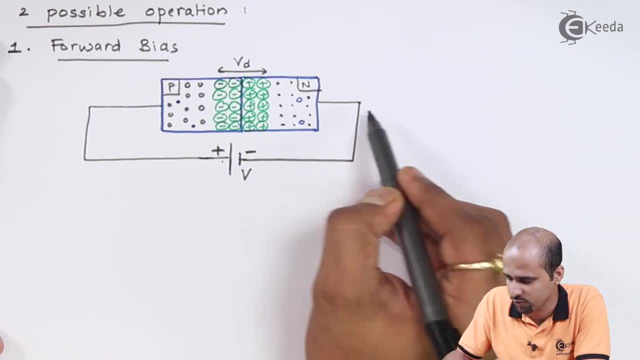 getting attracted towards this positive, getting attracted towards this positive. terminal of battery. terminal of battery. terminal of battery. so current will move. electrons will move. so current will move, electrons will move, so current will move. electrons will move towards this particular direction, towards this particular direction, towards this particular direction. electrons will move in this particular. 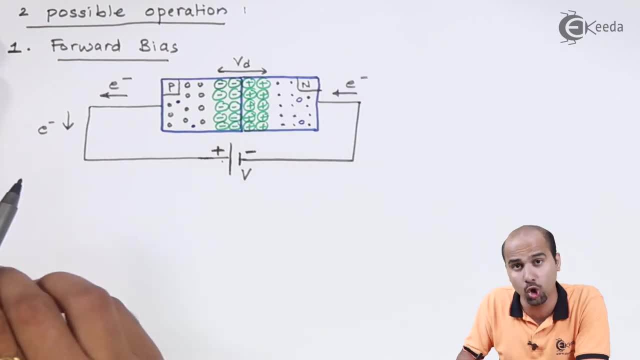 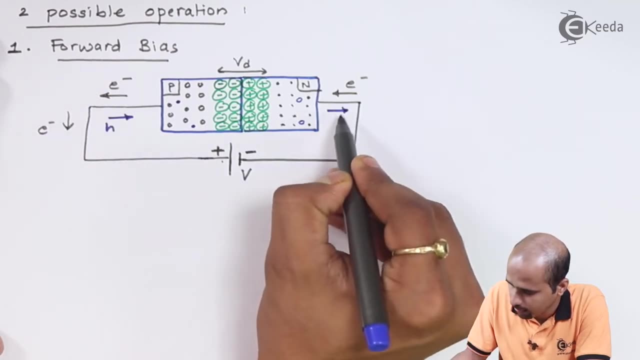 electrons will move in this particular electrons will move in this particular direction, direction, direction, and the holes and the holes and the holes will move in this particular direction. now, what is whole holes are nothing, but now, what is whole holes are nothing. but now, what is whole holes are nothing but the. 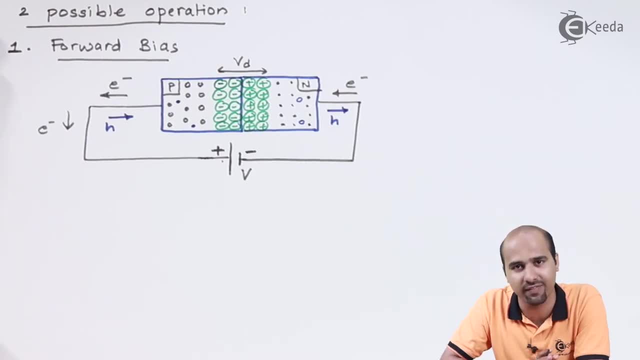 the the deficiency of electron empty chair. deficiency of electron empty chair. deficiency of electron empty chair and when it gets filled with the electron and when it gets filled with the electron and when it gets filled with the electron, that process is called as recombination. that process is called as recombination. 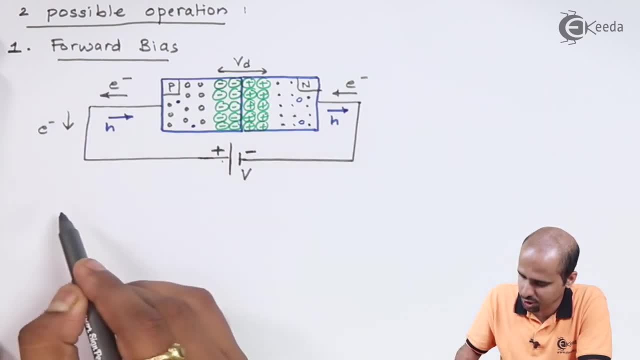 that process is called as recombination. okay, okay, okay, let's, let's, let's start, let's start, let's start the operation. this operation is called as the operation. this operation is called as the operation. this operation is called as forward bias. this is because the diode 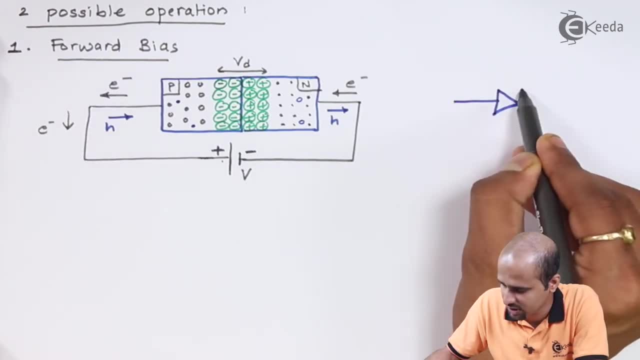 forward bias. this is because the diode forward bias. this is because the diode operation and symbol is concerned. this is operation and symbol is concerned. this is operation and symbol is concerned. this is nothing but the symbol of diode where, nothing but the symbol of diode where. 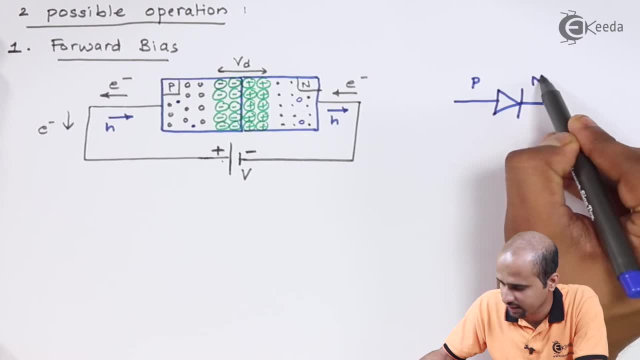 nothing but the symbol of diode, where this is nothing but the P type. this is nothing but the P type, this is nothing but the P type semiconductor and this is nothing but the semiconductor, and this is nothing but the semiconductor, and this is nothing but the n-type semiconductor. this is called as: 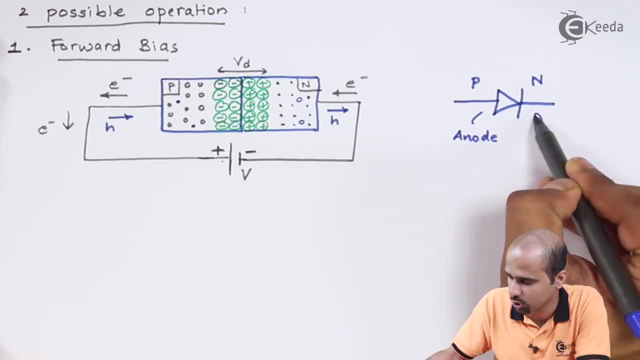 n-type semiconductor. this is called as n-type semiconductor, this is called as anode and this is called as cathode anode, and this is called as cathode anode, and this is called as cathode. current will flow from anode to cathode current will flow from anode to cathode. 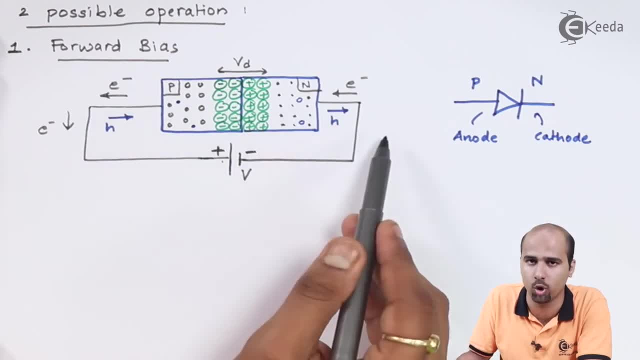 current will flow from anode to cathode as same as that of the direction of, as same as that of the direction of, as same as that of the direction of holes, and oppose it to the direction of holes and oppose it to the direction of holes and oppose it to the direction of conventional flow of the electron. so 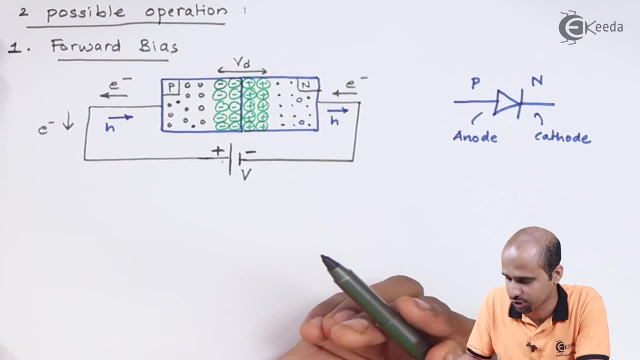 conventional flow of the electron, so conventional flow of the electron. so the conventional flow of current is exactly the conventional flow of current is exactly the conventional flow of current is exactly opposed to the flow of electron. so opposed to the flow of electron, so opposed to the flow of electron. so that's why this is called as forward. 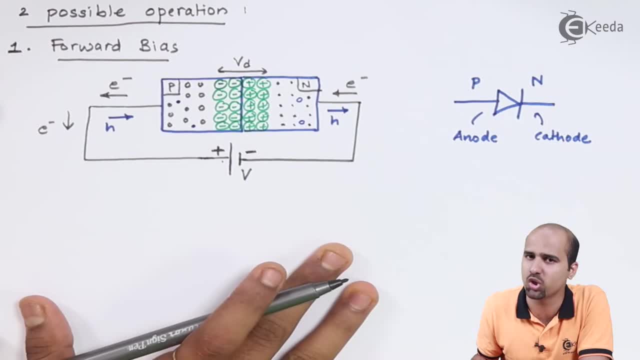 that's why this is called as forward. that's why this is called as forward bias. here I have kept my DC voltage bias. here I have kept my DC voltage bias. here I have kept my DC voltage constant. so whatever amount of energy constant. so whatever amount of energy. 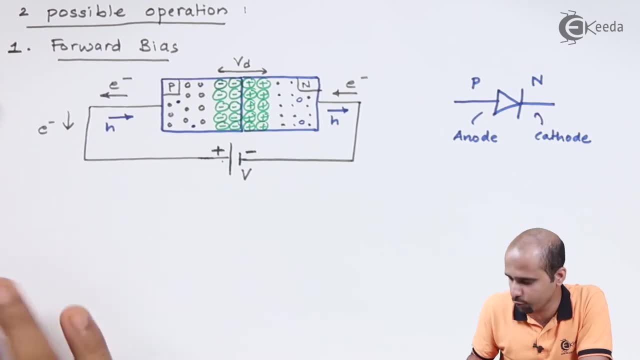 constant. so whatever amount of energy electrons gains and move towards the P electrons gains and move towards the P electrons gains and move towards the P channel and move towards the P type that channel and move towards the P type that channel and move towards the P type, that much amount of energy will get and will 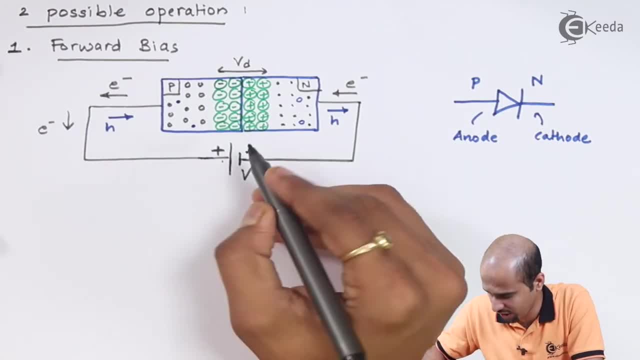 much amount of energy will get and will much amount of energy will get and will stop this operation right. but if I stop this operation right, but if I stop this operation right, but if I change this particular DC voltage, change this particular DC voltage, change this particular DC voltage towards the positive side, then this: 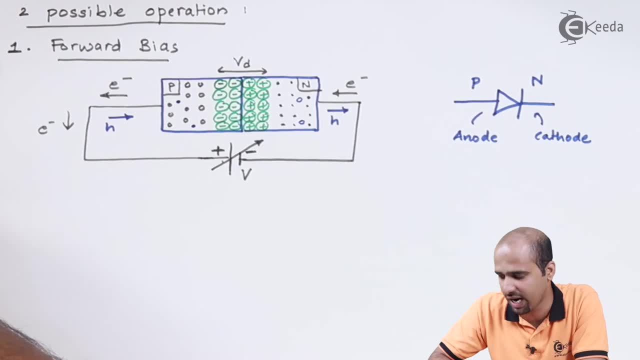 towards the positive side, then this towards the positive side, then this force will increase and increase and force will increase and increase, and force will increase and increase and increase and the electron velocity increase and the electron velocity increase and the electron velocity will increase more number of electrons. 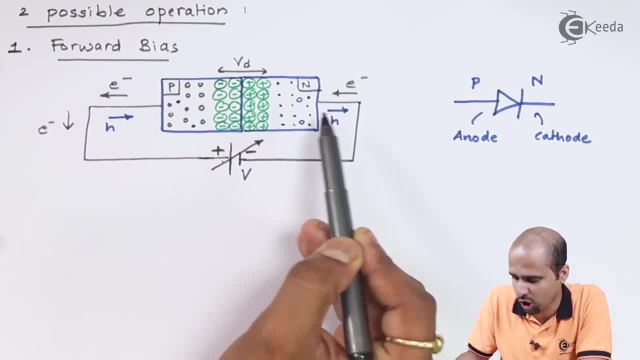 will increase. more number of electrons will increase. more number of electrons will cross the barrier. if more number of will cross the barrier, if more number of will cross the barrier, if more number of electrons crosses the barrier, then I can. electrons crosses the barrier, then I can. electrons crosses the barrier, then I can say that the current which forming in 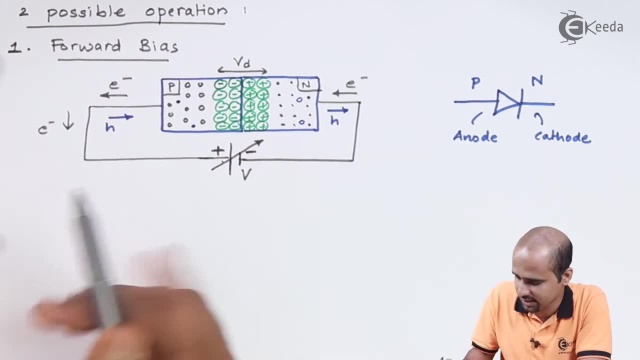 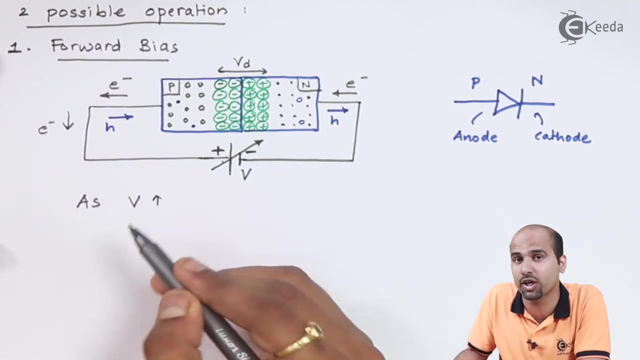 say that the current which forming in, say that the current which forming in this particular circuit will increase. so this particular circuit will increase. so this particular circuit will increase so as V increases the flow of electron, as V increases the flow of electron, as V increases the flow of electron, number of electrons passing through the 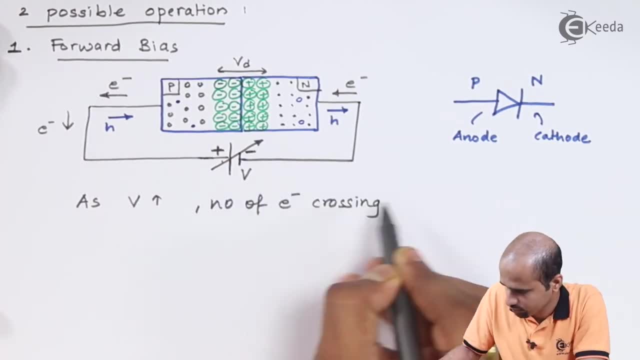 number of electrons passing through. the number of electrons passing through the junction increases. junction increases. junction increases. this increment of current is exponentially in the next, this increment of current is exponentially in the next, this increment of current is exponentially. in the next video we will clearly mention how that. 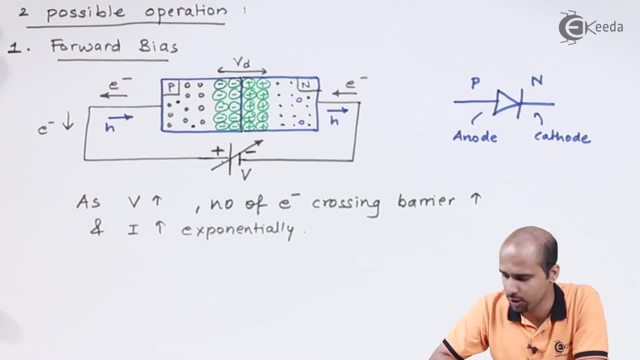 video. we will clearly mention how that video, we will clearly mention how that current increases exponentially, current increases exponentially, current increases exponentially mathematically as well. so as far as mathematically as well, so as far as mathematically as well, so as far as forward bias is concerned, I will get to. 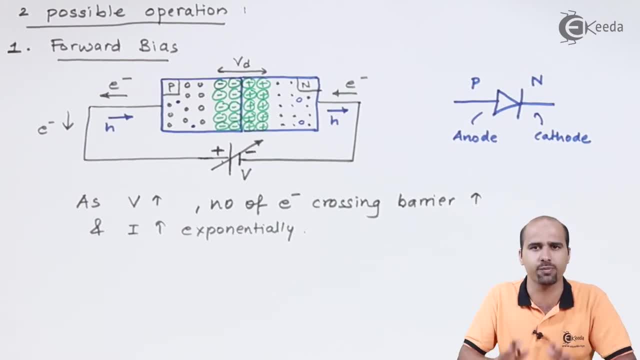 forward bias is concerned, I will get to. forward bias is concerned, I will get to know that if voltage increases current, know that if voltage increases current, know that if voltage increases current will increase exponentially due to the will increase exponentially due to the will increase exponentially due to the fact that electrostatic force of 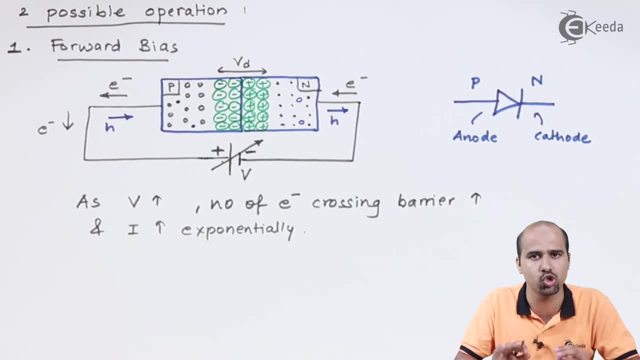 fact that electrostatic force of fact, that electrostatic force of attraction and repulsion will lead. attraction and repulsion will lead. attraction and repulsion will lead electrons to move from n-type to p-type, electrons to move from n-type to p-type, electrons to move from n-type to p-type, and holes to move from p-type to n-type. 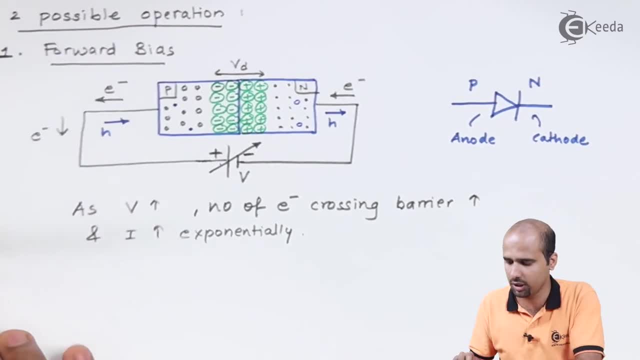 and holes to move from p-type to n-type and holes to move from p-type to n-type. exactly what operation we will learn in exactly what operation we will learn in exactly what operation we will learn in the next process that is called as. the next process that is called as: 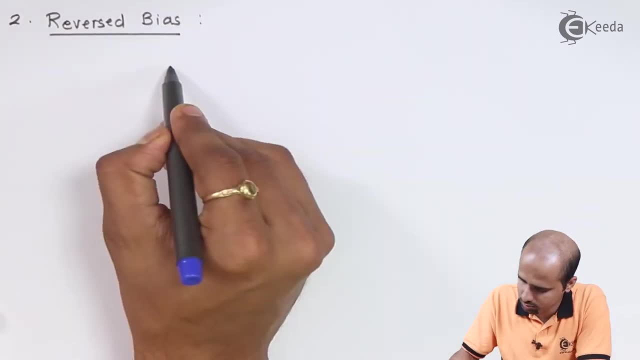 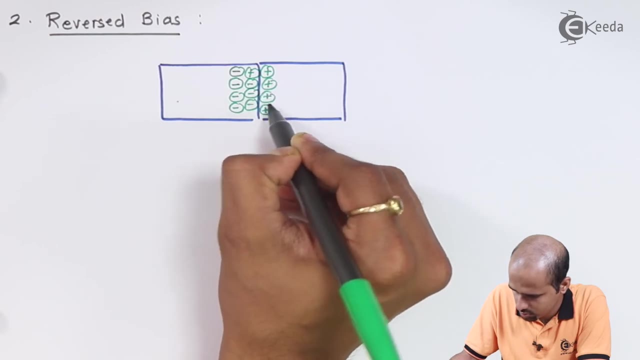 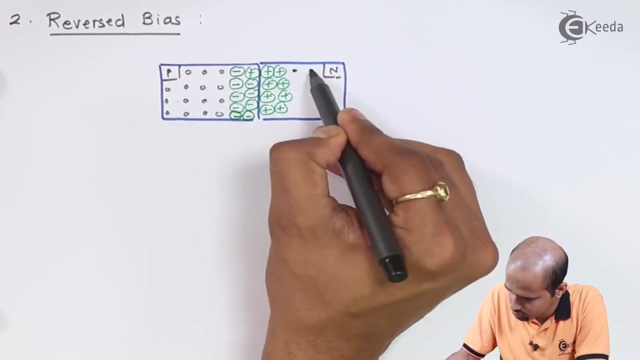 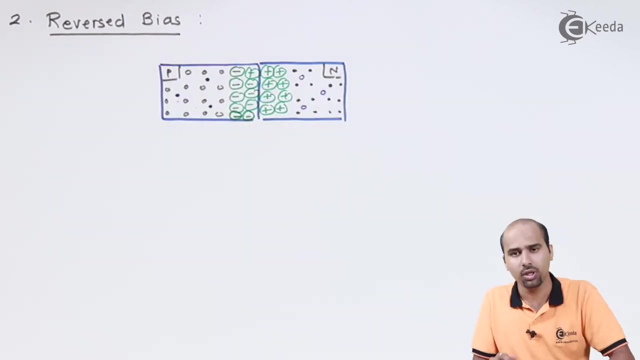 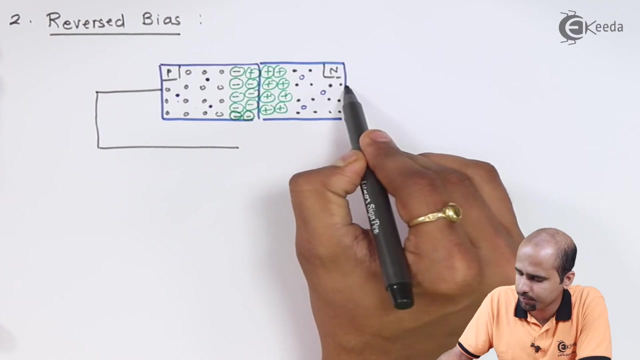 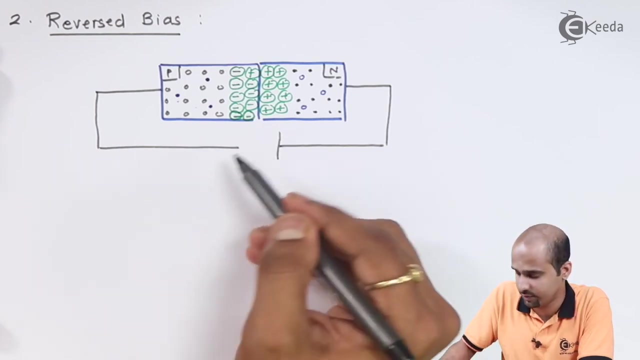 the next process that is called as reversed by us. now in this process, we will just apply the now in this process, we will just apply the now in this process, we will just apply the reverse polarity voltage supply. if you apply positive of battery towards. if you apply positive of battery towards. 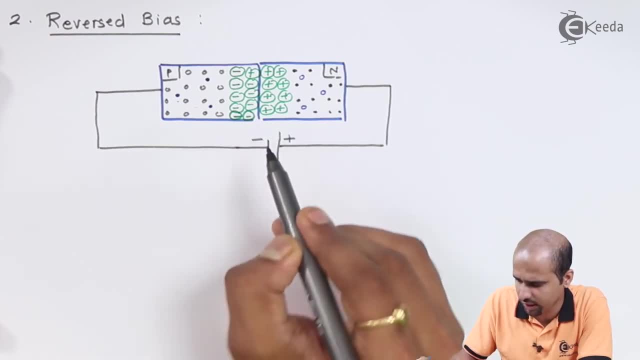 if you apply positive of battery towards the n-type, then what will happen? just the n-type? then what will happen? just the n-type? then what will happen? just analyze by using electrostatics force. analyze by using electrostatics force. analyze by using electrostatics force of attraction and repulsion. if we say 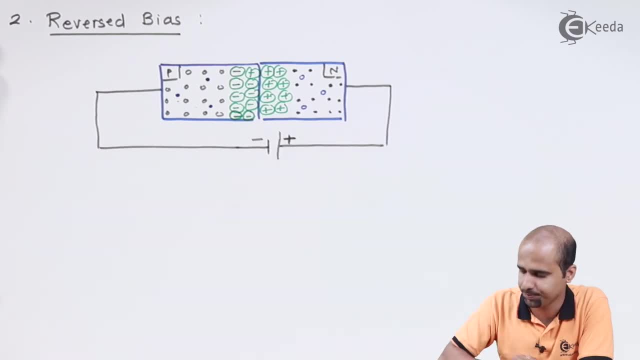 of attraction and repulsion. if we say of attraction and repulsion, if we say this is positively charged, terminal of this is positively charged. terminal of this is positively charged. terminal of battery which is connected to n-type of battery, which is connected to n-type of battery, which is connected to n-type of semiconductor and p-type of. 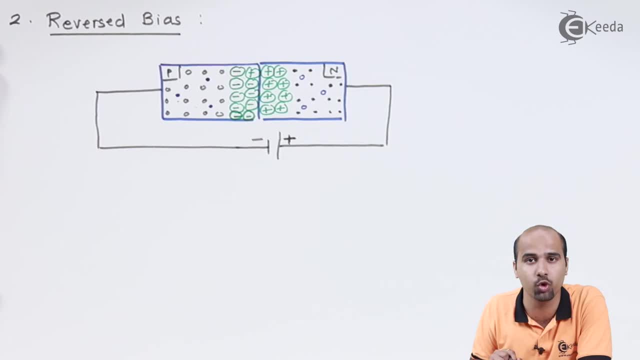 semiconductor and p-type of semiconductor. and p-type of semiconductor is connected to negative. semiconductor is connected to negative. semiconductor is connected to negative. what will happen? attractive force will. what will happen, attractive force will. what will happen, attractive force will get developed. now we can say these: get developed. now we can say these. 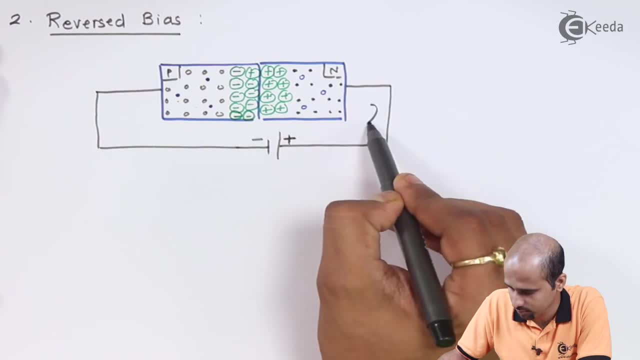 get developed. now we can say: these electrons will move towards the electron electrons will move towards the electron electrons will move towards the electron movements is towards the positive type movements is towards the positive type movements is towards the positive type of battery and holes. movement is towards of battery and holes movement is towards 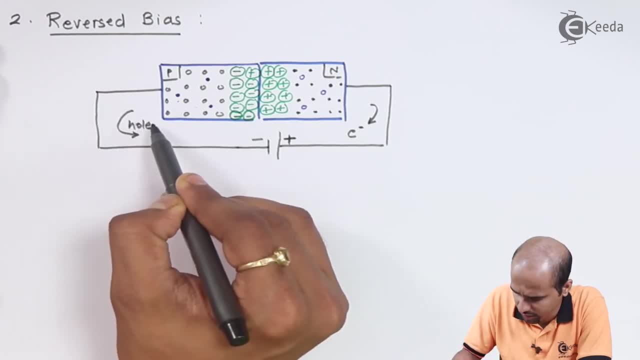 of battery and holes. movement is towards the negative type of battery. right then, the negative type of battery. right then, the negative type of battery. right then. what will happen? just say he holds p. what will happen? just say he holds p. what will happen? just say he holds p types of our nickel there. just say: 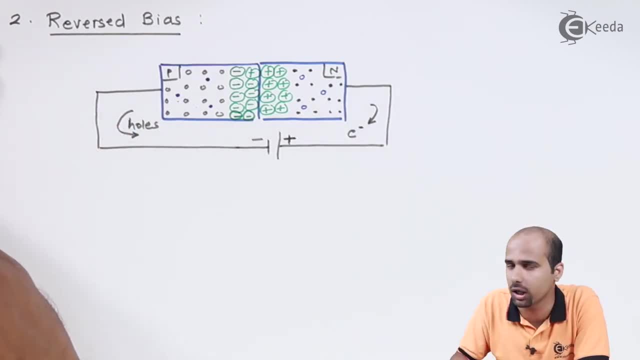 types of our nickel. there just say types of our nickel. there just say electrons and types of our nickel. there: electrons and types of our nickel. there, electrons and types of our nickel. there atom will get converted into ions. so atom will get converted into ions. so atom will get converted into ions. so what will happen as the electrons are? 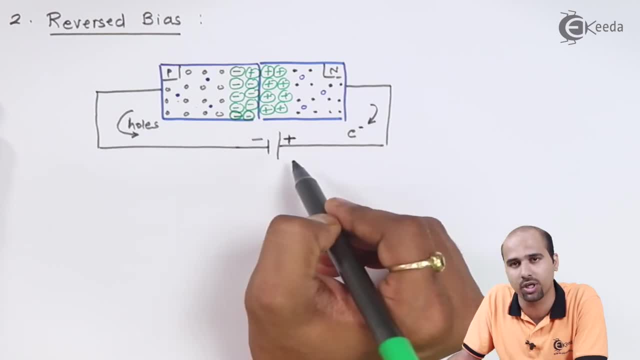 what will happen as the electrons are? what will happen as the electrons are moving from n-type to positive terminal, moving from n-type to positive terminal, moving from n-type to positive terminal, of battery and P holes from p-type to of battery and P holes from p-type to. 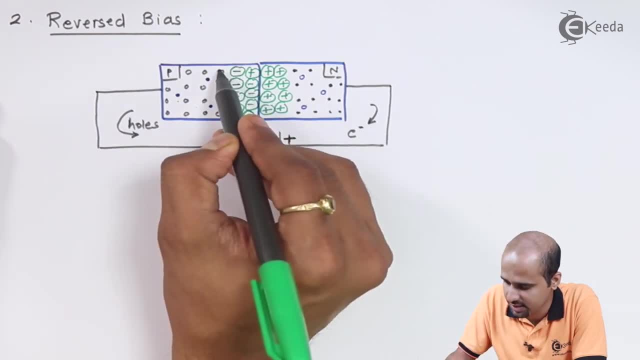 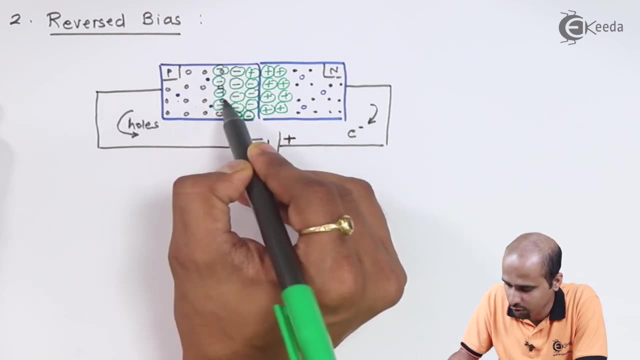 of battery and P holes from p-type to negative terminal of battery, then I can negative terminal of battery, then I can negative terminal of battery, then I can say that this will get converted into, say that this will get converted into, say that this will get converted into ions. so what we have observed, we have 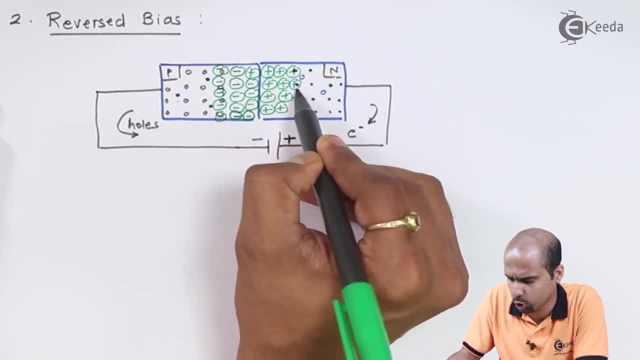 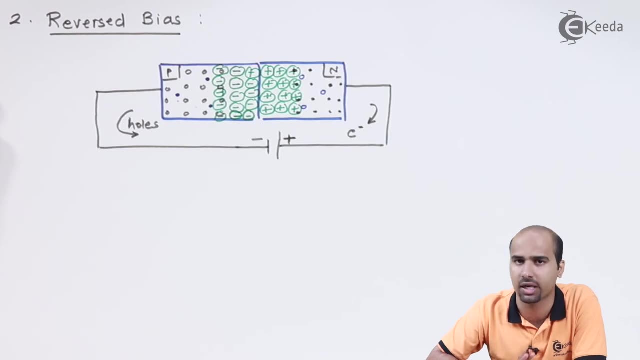 ions. so what we have observed: we have ions. so what we have observed: we have observed that atoms are converted into observed, that atoms are converted into observed, that atoms are converted into positive and negatively charged ions, in positive and negatively charged ions, in positive and negatively charged ions, in n-type and p-type semiconductor. 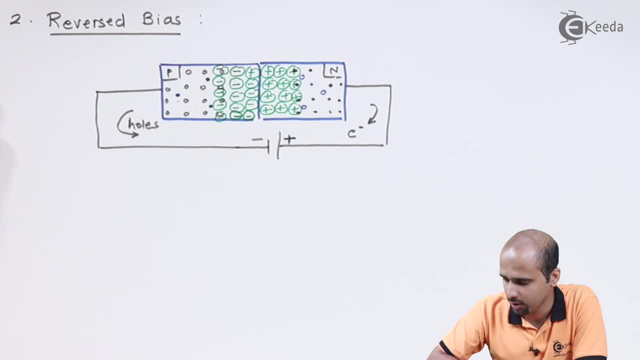 n-type and p-type semiconductor. n-type and p-type semiconductor, respectively in the construction of diode, respectively in the construction of diode, respectively in the construction of diode. right. so what will happen? this right? so what will happen? this right? so what will happen? this width will get increased if width increases. 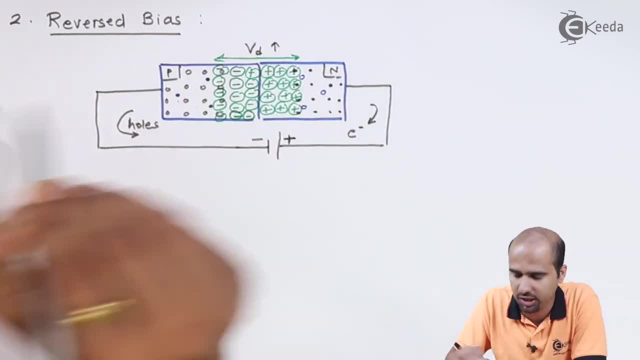 width will get increased if width increases. width will get increased if width increases, then can I say that this potential will. then can I say that this potential will, then can I say that this potential will get increased. then the resistance which get increased, then the resistance which get increased, then the resistance which is nothing but the resistive power to. 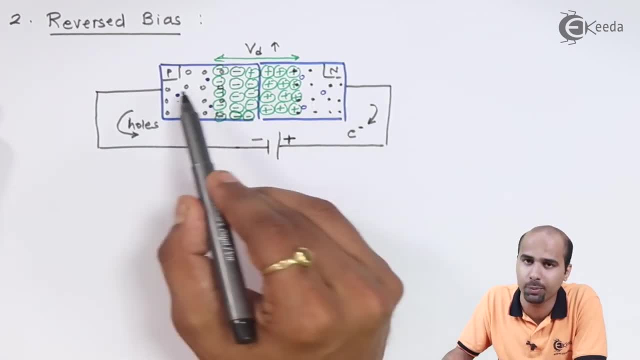 is nothing but the resistive power to is nothing but the resistive power to resist the electrons to move from n-type. resist the electrons to move from n-type. resist the electrons to move from n-type to p-type is increasing. we can say the to p-type is increasing. we can say the. 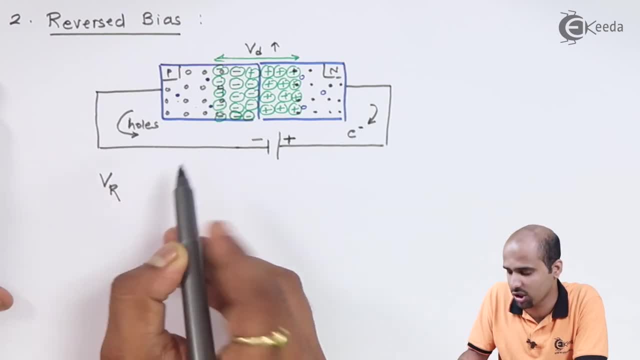 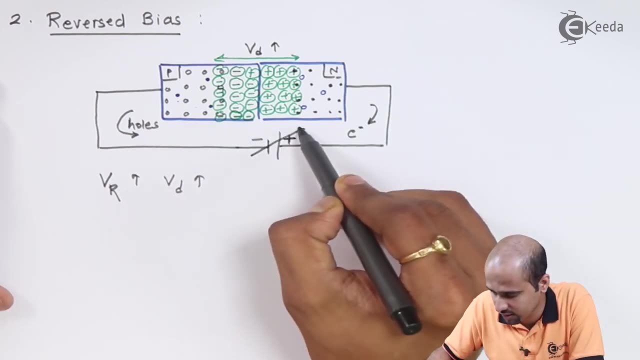 to p-type is increasing. we can say: the VR resistor across this junction is VR resistor across this junction is VR resistor across this junction is increases. V D increases if we increase increases. V D increases if we increase increases. V D increases if we increase the value of this external potential. 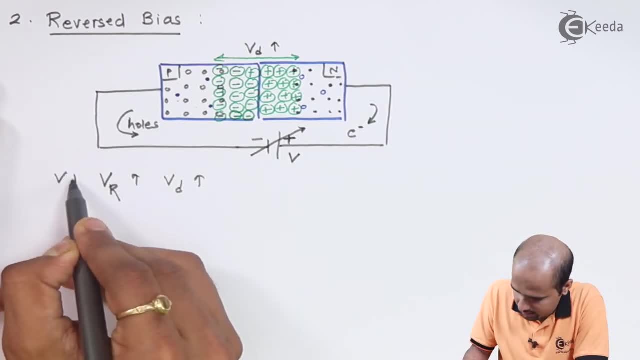 the value of this external potential, the value of this external potential power supply. if we increases, then we are power supply. if we increases, then we are power supply. if we increases, then we are increases. this V? D increases we can also increases. this V D increases we can also. 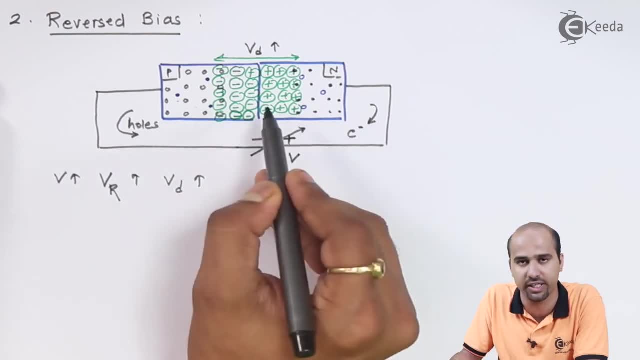 increases, this V D increases. we can also say that this distance increases. is say that this distance increases is say that this distance increases is proportional with the V D. now, what will proportional with the V D now? what will proportional with the V D now, what will happen? can I say that there will not be. 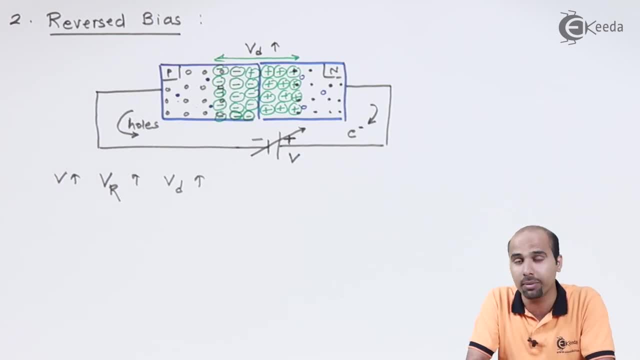 happen? can I say that there will not be happen? can I say that there will not be any flow of current? yes, there will not be any flow of current. yes, there will not be any flow of current. yes, there will not be any flow of current. ideally, but don't. 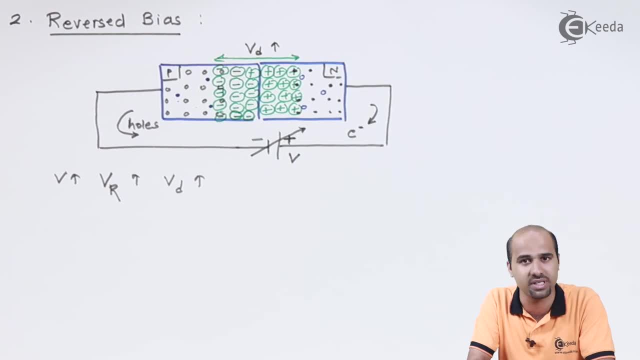 any flow of current, ideally, but don't any flow of current, ideally. but don't neglect all the minority charge carrier. neglect all the minority charge carrier. neglect all the minority charge carrier I have represented. see this minority I have represented. see this minority I have represented. see this minority charge carriers. electron, electron and. 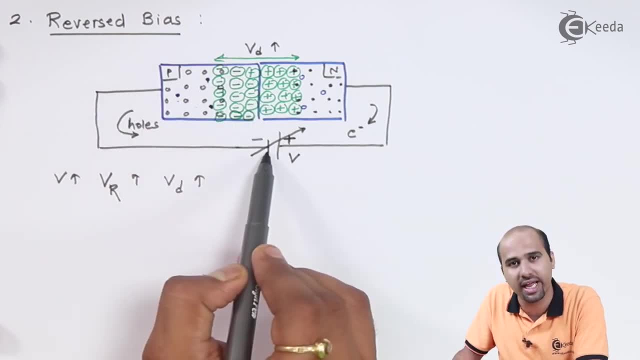 charge carriers electron- electron and charge carriers electron, electron and electron. I have connected this P type to electron. I have connected this P type to electron. I have connected this P type to negatively charged terminal of power. negatively charged terminal of power, negatively charged terminal of power supply and positively charge correct is. 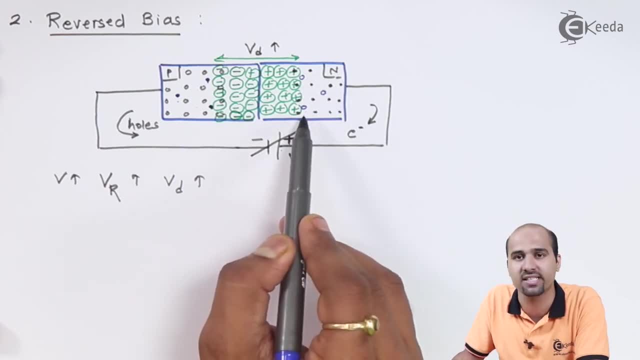 supply and positively charge correct. is supply and positively charge correct. is connected to n type n type memory pass. connected to n type n type memory pass. connected to n type n type memory pass. holes here as minority charge carriers now. holes here as minority charge carriers now. holes here as minority charge carriers: now this minority charge carrier is. 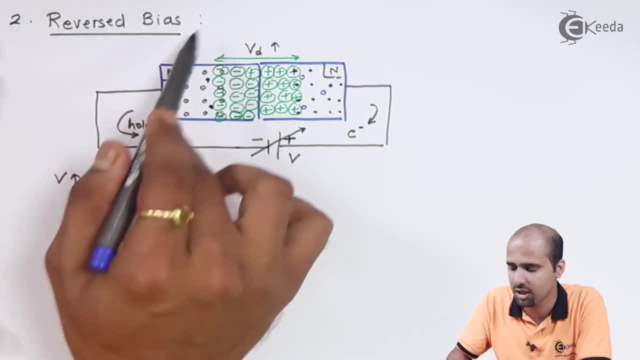 this minority charge carrier? is this minority charge carrier is responsible for this conduction process? responsible for this conduction process? responsible for this conduction process under the reverse bias operation, now in under the reverse bias operation, now in under the reverse bias operation, now in the reverse bias operation. these 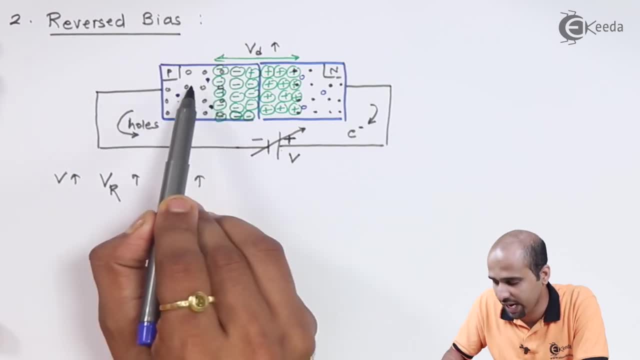 the reverse bias operation, these, the reverse bias operation, these minority charge carriers. what will minority charge carriers? what will minority charge carriers? what will happen? this will try to enter into the happen. this will try to enter into the happen. this will try to enter into the junction barrier if they get sufficient. 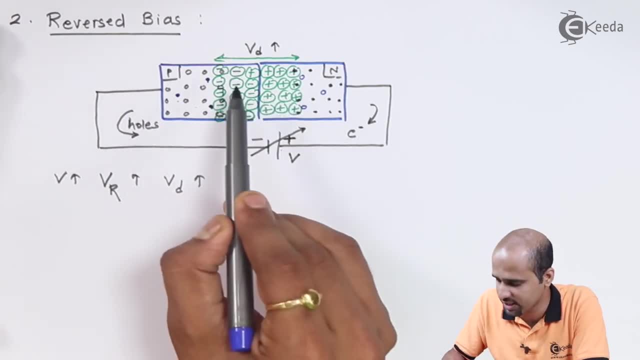 junction barrier. if they get sufficient junction barrier, if they get sufficient amount of energy to break the covalent amount of energy, to break the covalent amount of energy, to break the covalent bond, then obviously this will jump bond. then obviously this will jump. 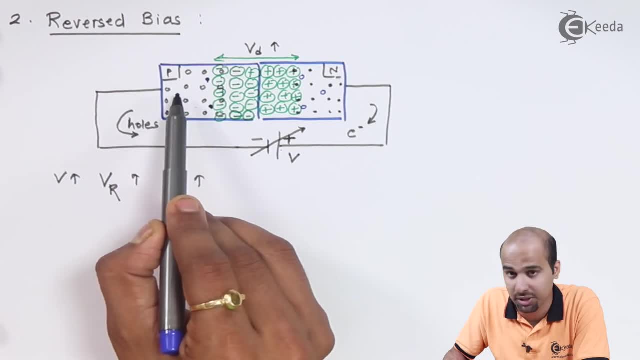 bond, then obviously this will jump towards the n type. and if electrons in towards the n type and if electrons in towards the n type, and if electrons in the p-type move towards the n-type, then the p-type move towards the n-type, then the p-type move towards the n-type, then flow of electron will be from here when 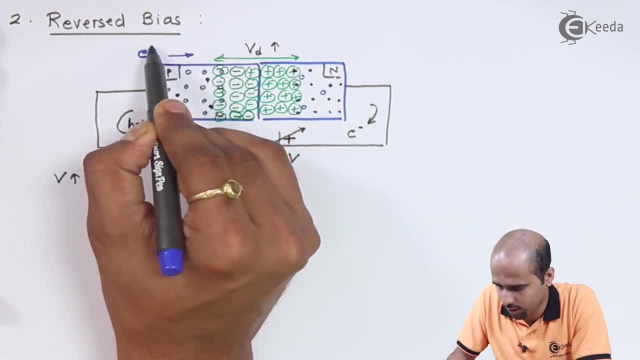 flow of electron will be from here. when flow of electron will be from here. when flow of minority charge electrons will flow of minority charge electrons will flow of minority charge electrons will be from here. em is nothing but the be from here. em is nothing but the be from here. em is nothing but the minority charge electrons. so electrons. 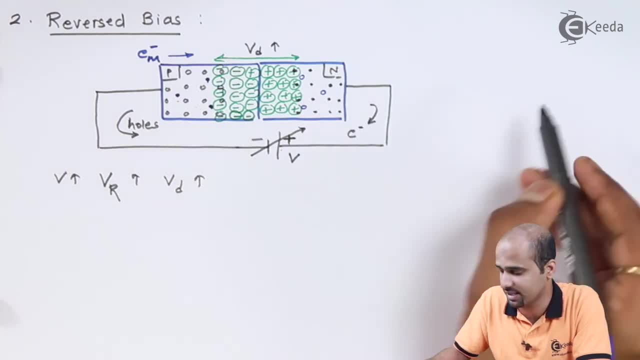 minority charge electrons, so electrons minority charge electrons, so electrons will move from p-type to n-type and I will move from p-type to n-type and I will move from p-type to n-type. and I can say that as far as this diode symbol can say that, as far as this diode symbol. 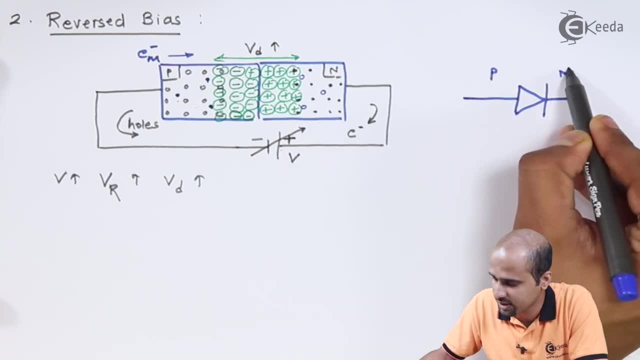 can say that, as far as this diode symbol is concerned, we will say this is p-type is concerned. we will say this is p-type is concerned. we will say this is p-type, this is n-type if electrons are moving. this is n-type if electrons are moving. 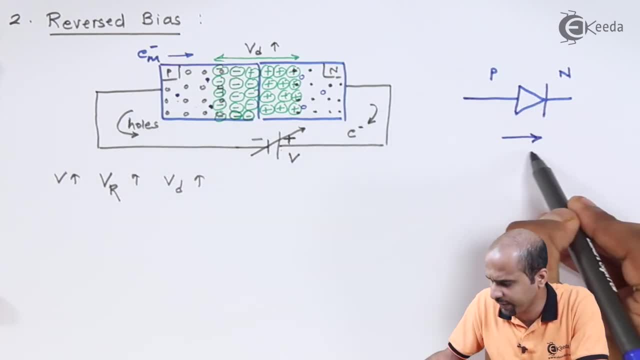 this is n-type if electrons are moving from. if electrons are moving from p-type from. if electrons are moving from p-type from. if electrons are moving from p-type to n-type minority charge carrier to n-type minority charge carrier to n-type minority charge carrier. electrons are moving from p-type to n-type. 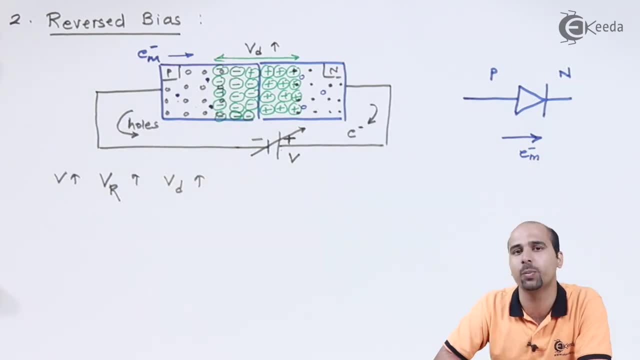 electrons are moving from p-type to n-type. electrons are moving from p-type to n-type, then conventional current will flow. then conventional current will flow. then conventional current will flow from n type to p-type, but mine will as this: from n type to p-type, but mine will as this: 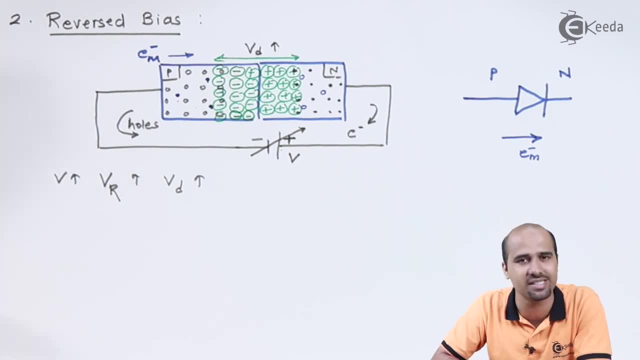 from n type to p-type, but mine will as this: minority charge carrier carriers are minority charge carrier carriers are minority charge carrier carriers are very, very less in numbers. so the very, very less in numbers. so the very, very less in numbers. so the movement and number of electrons passing. 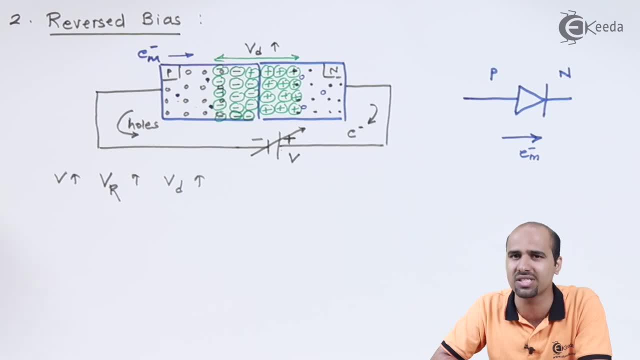 movement and number of electrons passing. movement and number of electrons passing through the Junction are very, very less through the Junction are very, very less. through the Junction are very, very less. if these numbers are very, very less, as if these numbers are very, very less, as if these numbers are very, very less as compared to majority charge carriers. 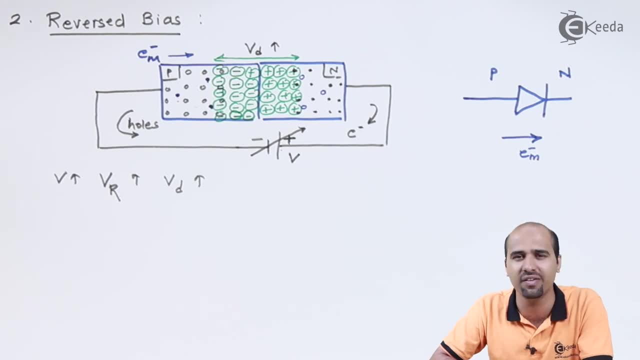 compared to majority charge carriers. compared to majority charge carriers, then whatever current I will be getting, then whatever current I will be getting, then whatever current I will be getting will be very, very less, but in opposite will be very, very less but in opposite will be very, very less, but in opposite direction. so current will move in.